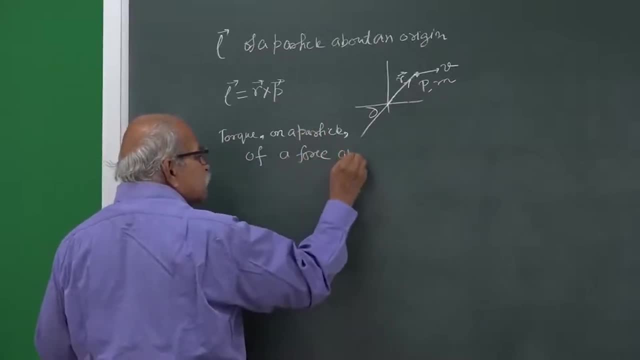 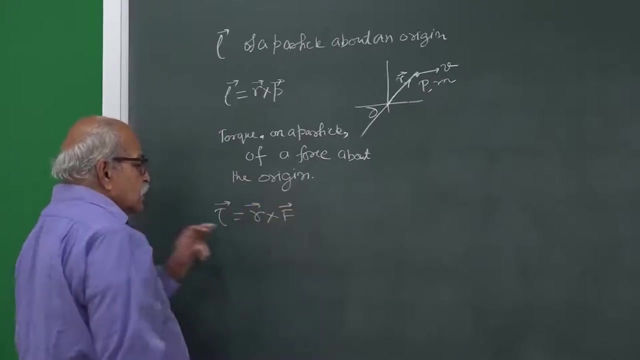 is acting on some particle, And once again, about the origin, about the origin. So this is important. And then we say that torque is r cross f. This r is same as this r. This is the position vector of the particle on which this force is acting And this position vector is taken. 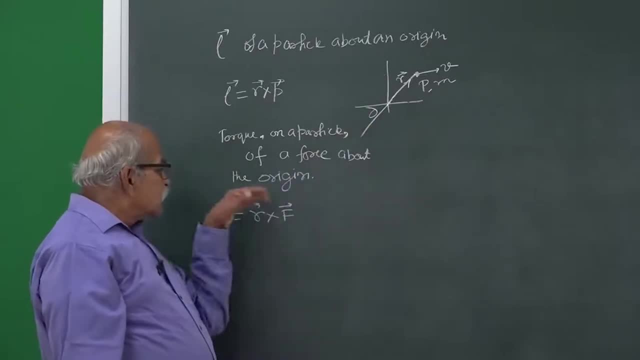 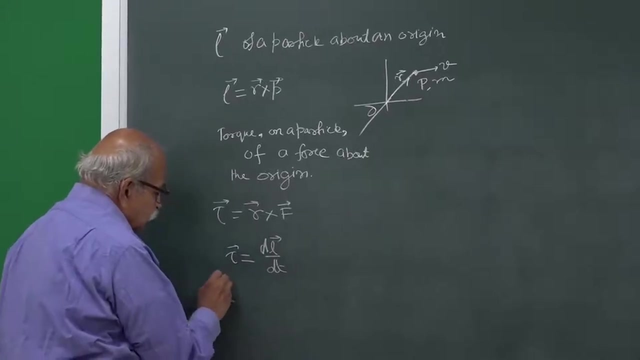 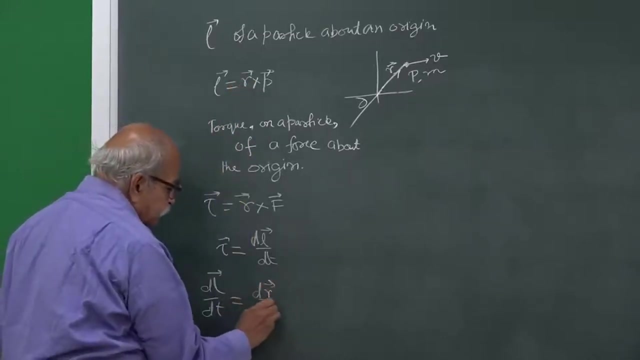 from the same origin and then we call this torque, about that point. and then you have a very simple relation: that torque is equal to dL by dt. dL by dt is simple L, you know. so dL by dt, if you do, it will be differentiation of the first function, cross, the second function. 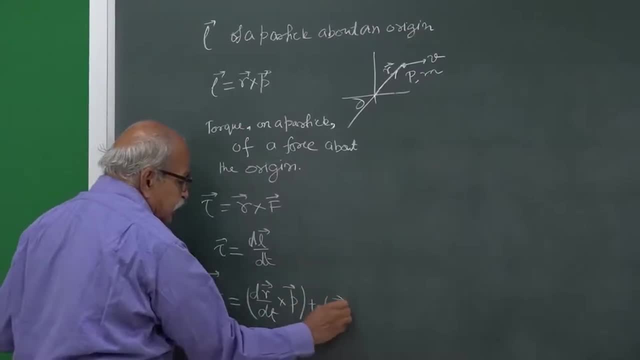 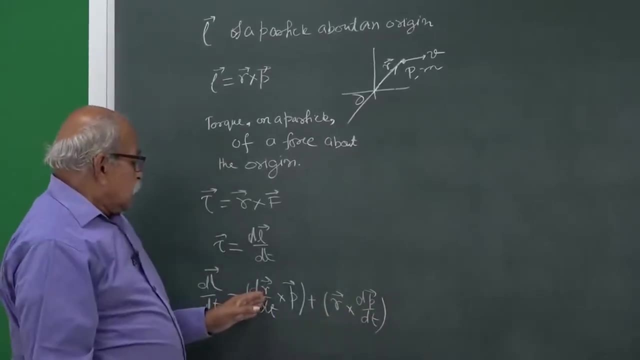 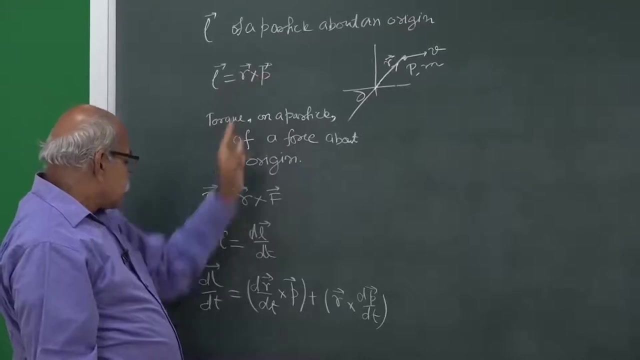 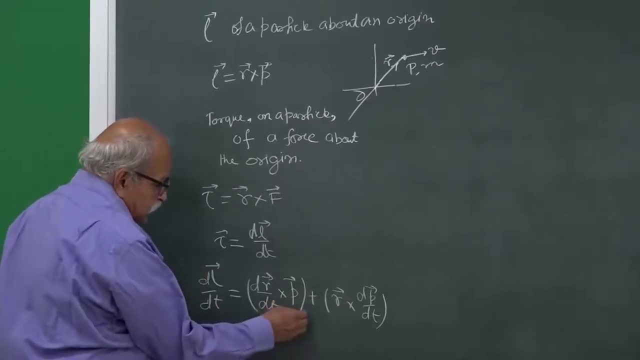 as such and then first function as such, and differentiation of this second vector. Now it is important that the order is not changed: r first, p next, r first, p next, r first, p next. order should not change. and then one sees that this is 0,. this is 0, why? 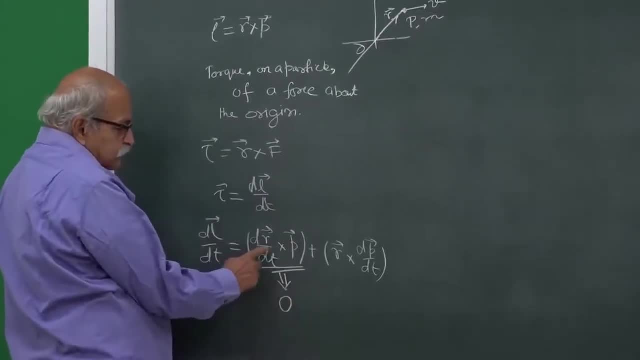 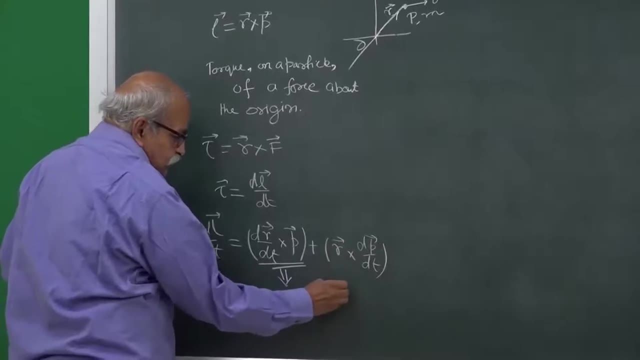 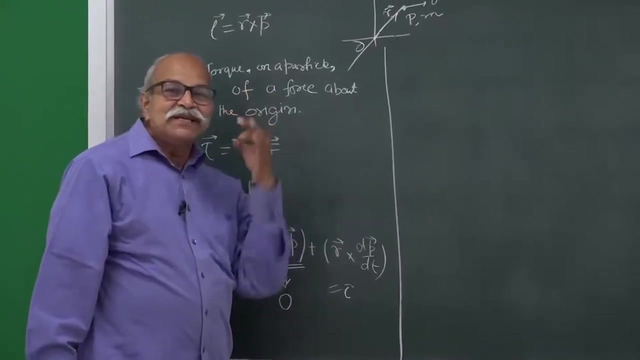 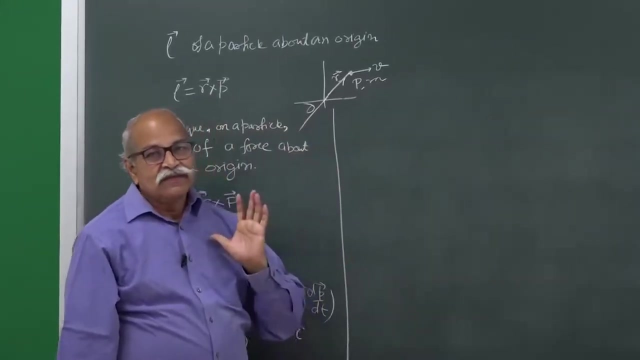 This is parallel to velocity, This is velocity itself, This is 0 and this is force, This is force, resultant force. dp, dt, and therefore this is equal to torque. simple. Now let me take a very common example. simple example: a particle freely falling under gravity. 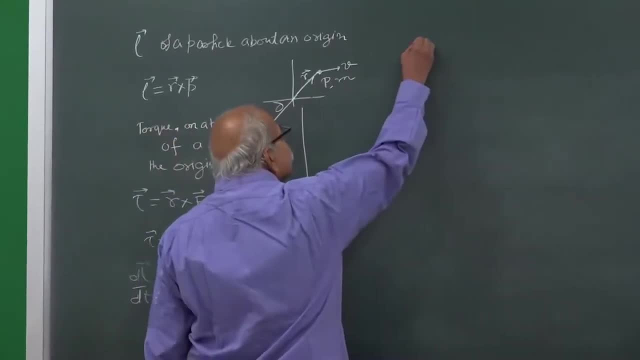 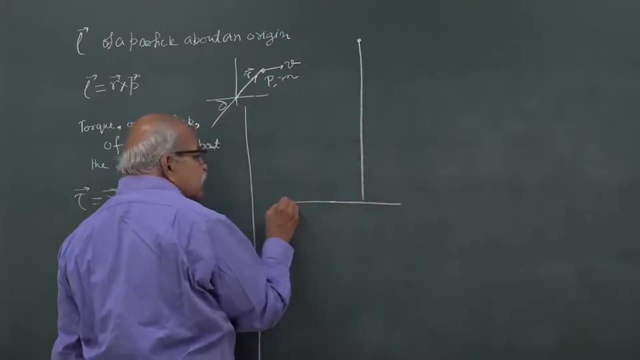 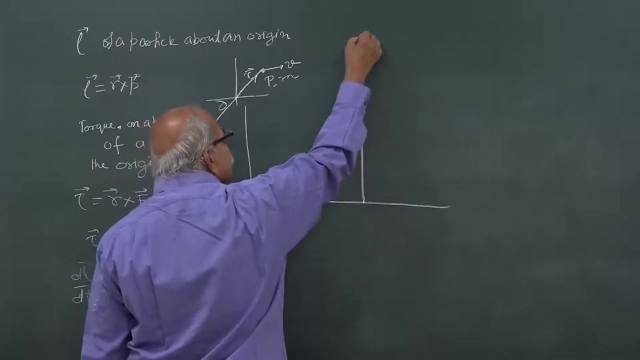 So it is dropped. a particle is dropped and then it falls. So it falls in a vertical line, It falls in a vertical line and then it reaches ground. It reaches ground, So it is dropped from here and we can take the origin right here and then x-axis, y-axis. 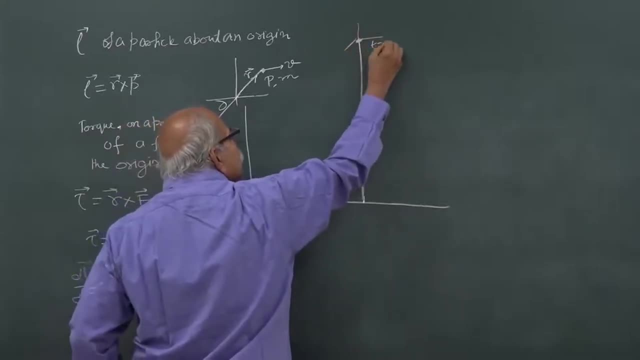 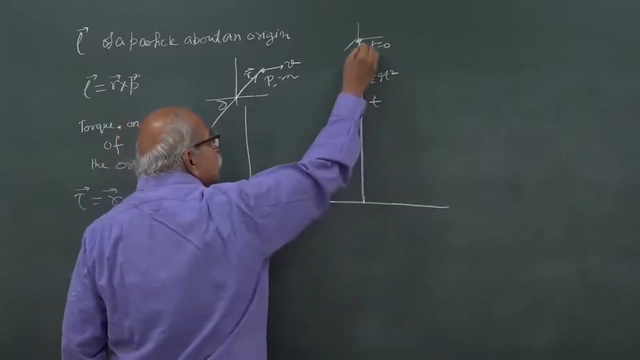 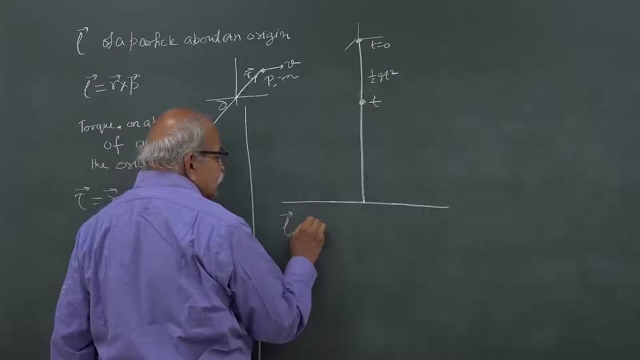 and z-axis, and if this time is t equal to 0, at certain time t it will be here. So this is at time t and this distance is half gt square, Okay, Okay. So if I ask, what is the angular momentum of this particle? at time t, so l, at time t. 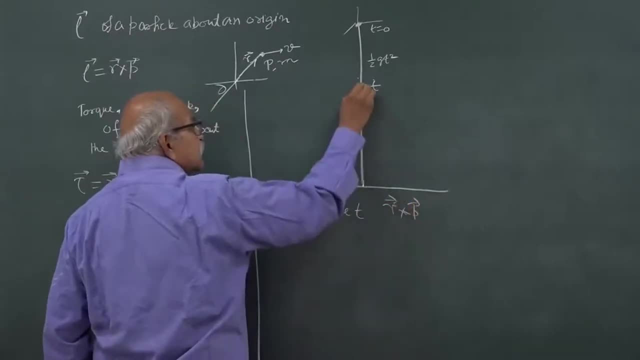 This is r cross p. Now what is the r vector? here is the origin. so this is our r vector, this is our position vector of the particle at time t. And what is the linear momentum? It is mass. It is mass. 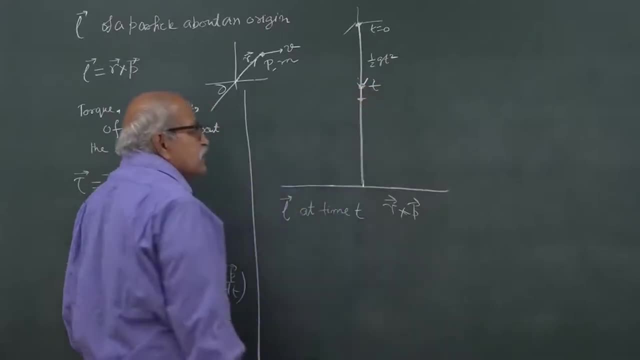 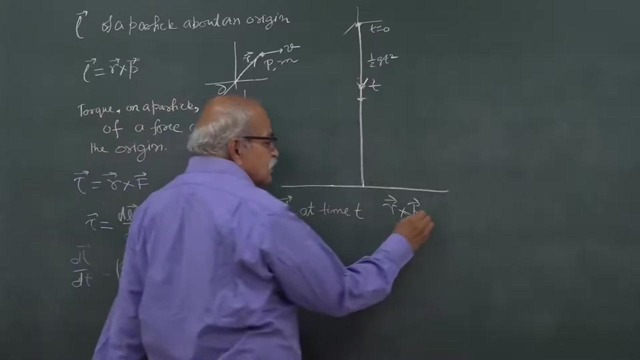 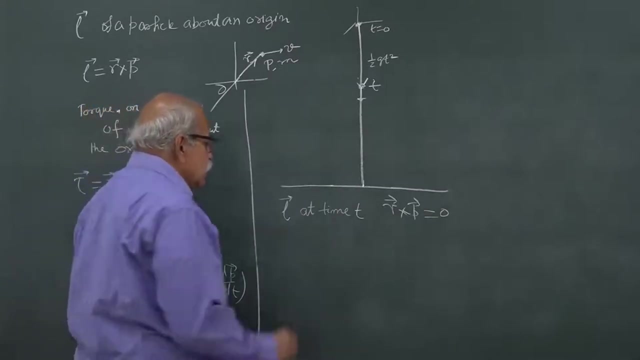 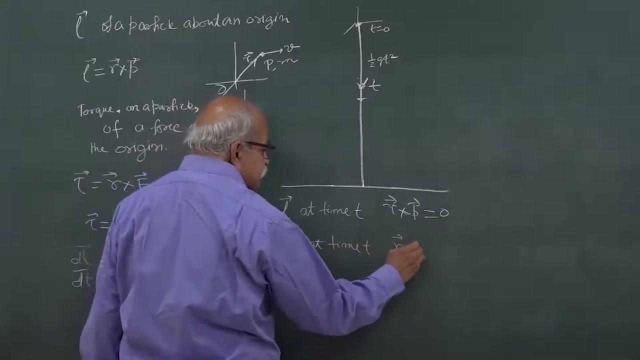 It is mass times velocity, mass times velocity, And the two are in the same direction. r vector and this p vector are in the same direction and therefore this is 0.. Angular momentum remains 0, it moves on this straight line And torque, torque at time t r cross f. that also you can work out. 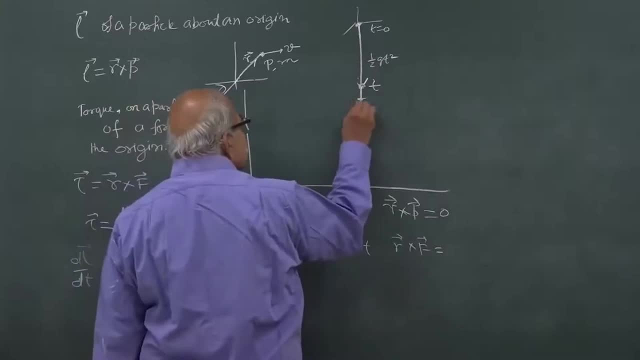 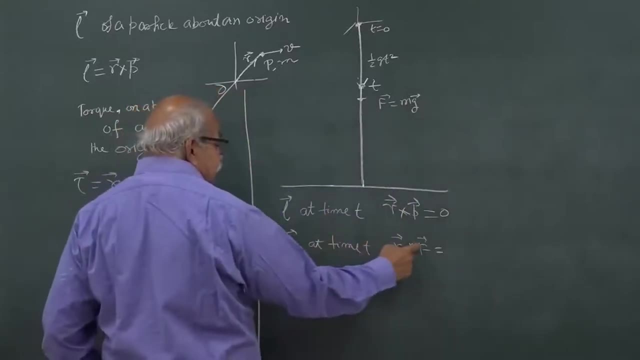 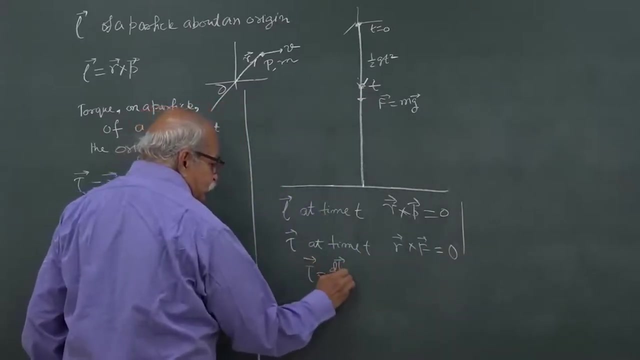 What is the force? The force is mg. The force is f. is mg which direction? vertically downward. So once again, r and f are parallel to each other and therefore it is 0.. So obviously, torque is dldt. l is 0 all the time. torque is 0 all the time, so torque. 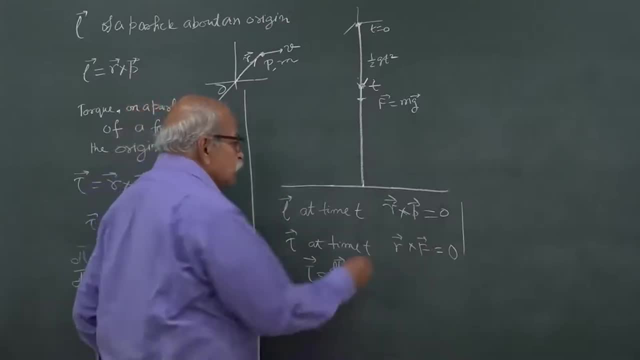 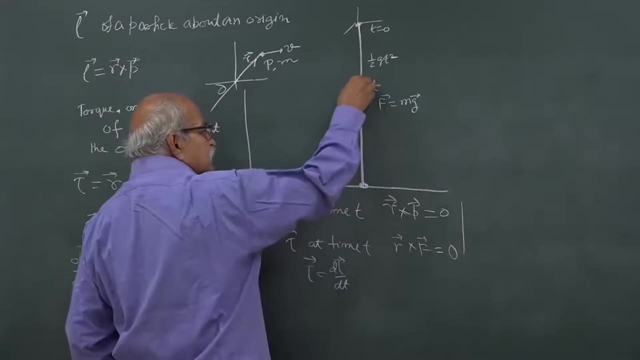 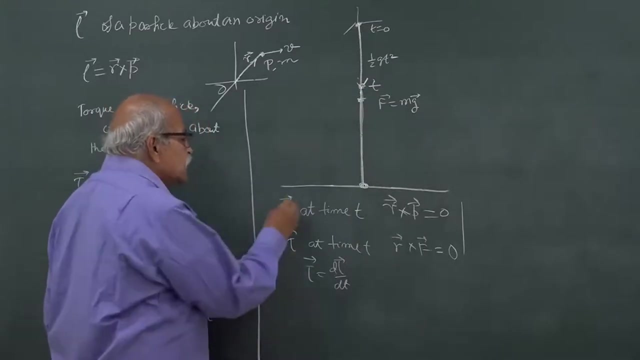 is dldt. so obviously correct If you take your origin here. same story, same story. this is r vector. This is r vector then, and this is f vector and this is p vector. so same story. What if I take the origin somewhere here? 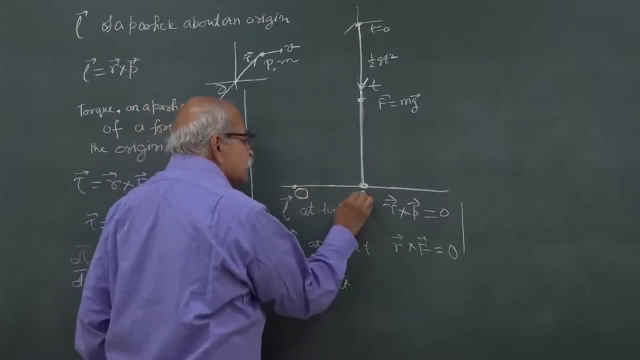 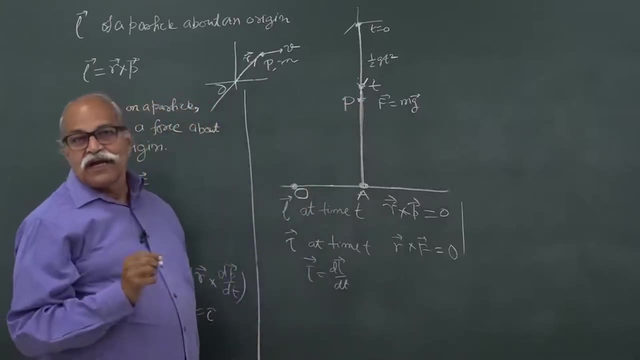 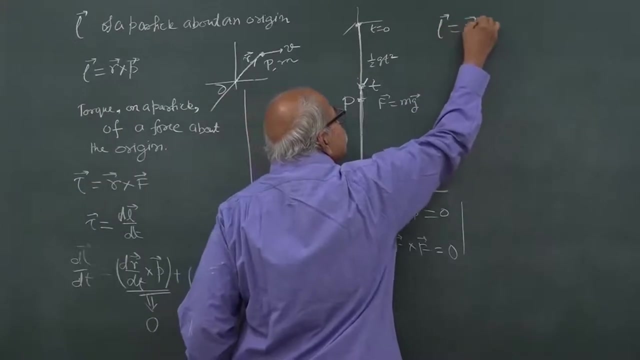 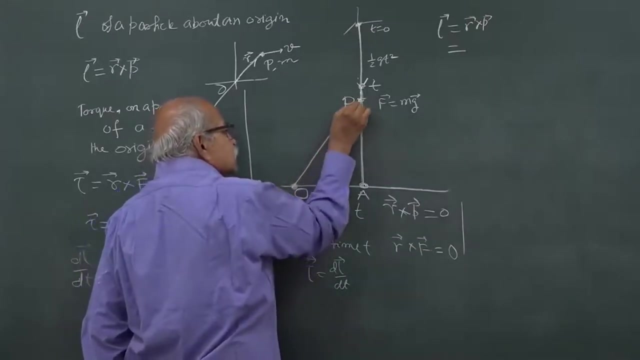 Let us say: this is a point O and this is point A and this is point P, and my origin is here. Now, what is the angular momentum? Is it 0?? The angular momentum l is r cross, p, r cross, p and r vector is from the origin to the particle. 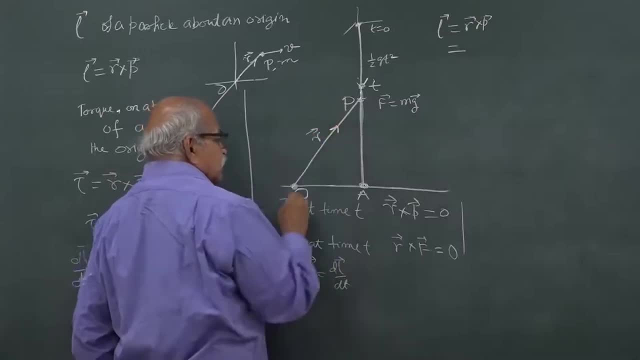 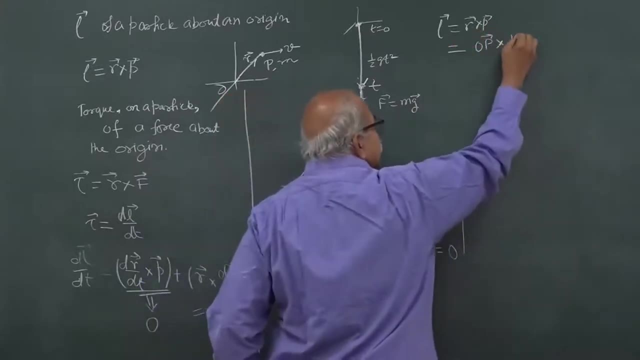 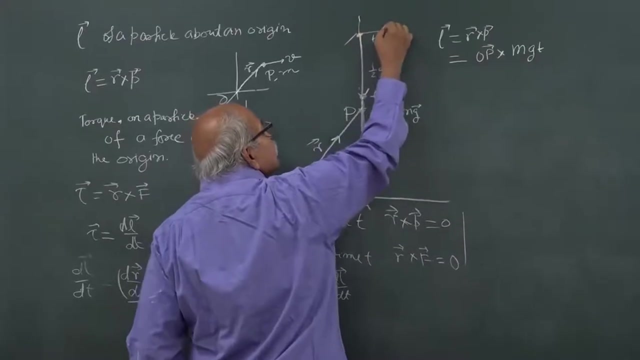 So this is r vector. So this is r vector op op cross product with p vector: mass times velocity. What is velocity gt? if I call this, let us say: this is x axis, this is y axis. 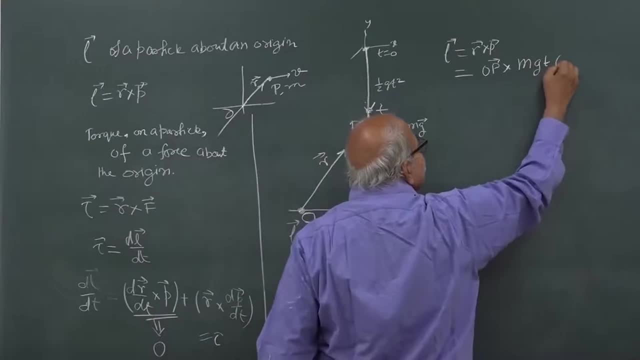 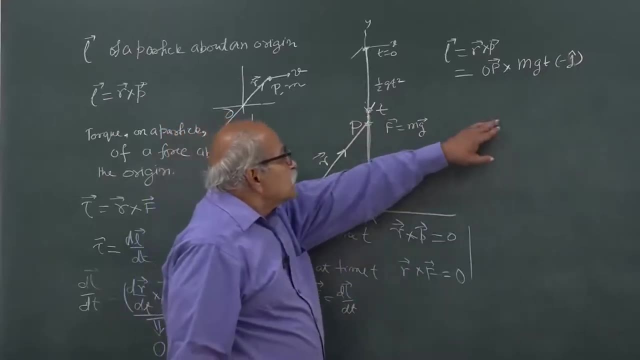 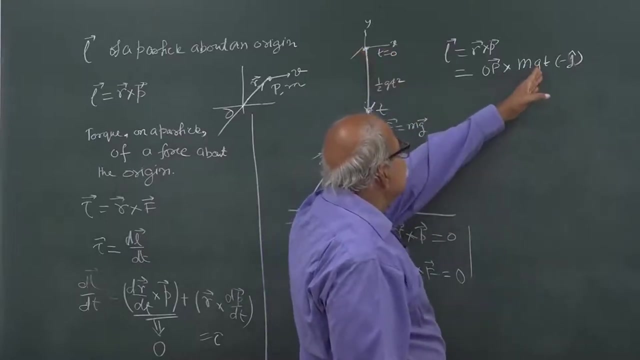 Then it is: velocity is gt. What is velocity? gt? gt in minus k cap direction, minus j cap direction. Velocity is g into t v equal to u plus gt. u is 0 and therefore it is mgt mass times. 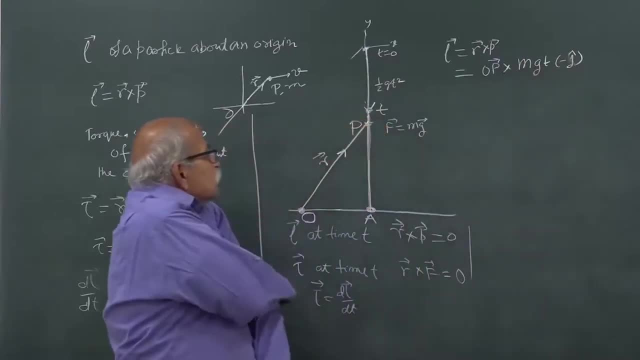 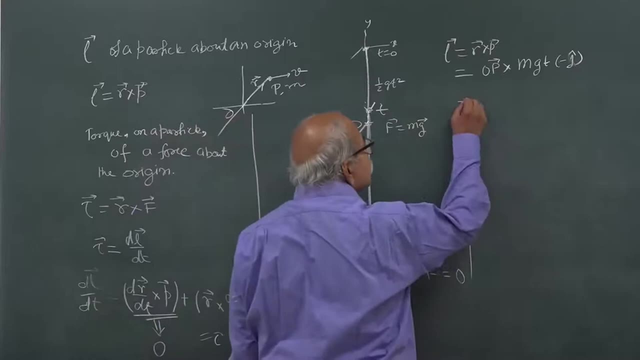 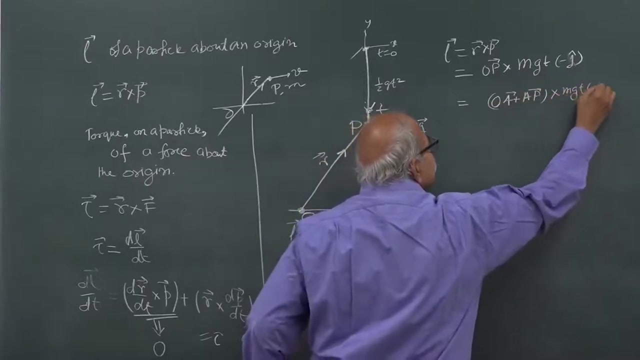 velocity and then the direction of the velocity is in minus j cap direction And if I work it out, this op vector is oa vector plus gt, So it is oa vector and plus ap vector And cross mgt and then minus j cap. 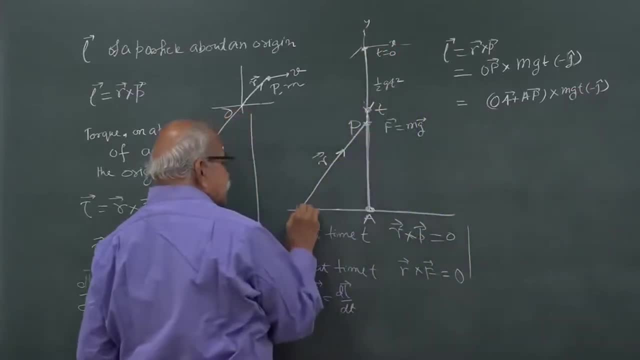 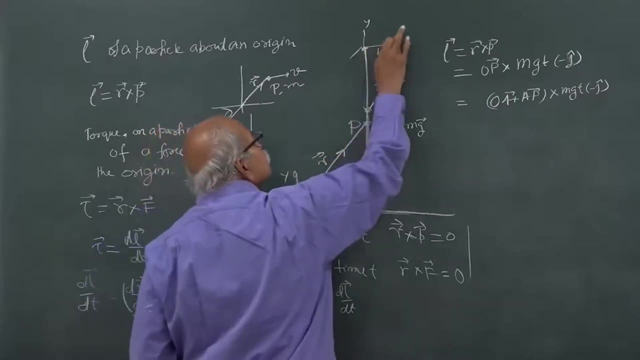 oa. this is x direction, So let us take origin here and this is our x direction. This is our y direction and the z direction is here. So this was earlier All right. So this is origin. This is the op vector. 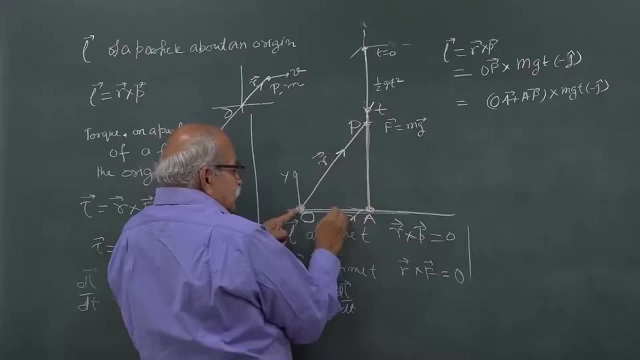 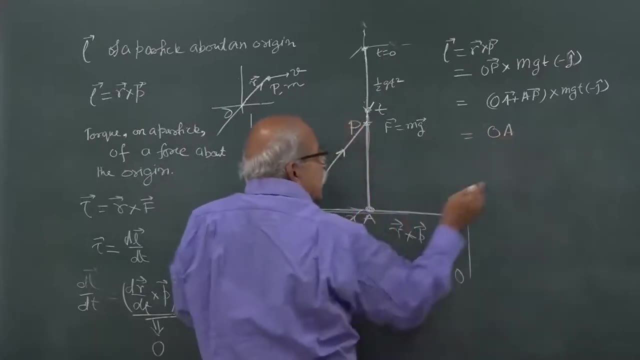 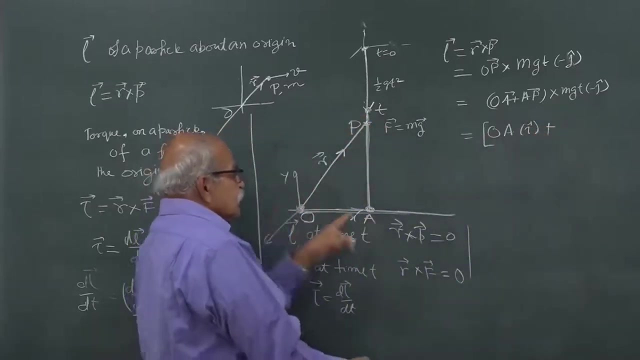 And which is We are writing oa plus ap. oa is this distance, This distance is some distance oa. So this is oa times and i cap, i cap plus ap, ap, ap. So it is ap, it is ap and times this what j vector. 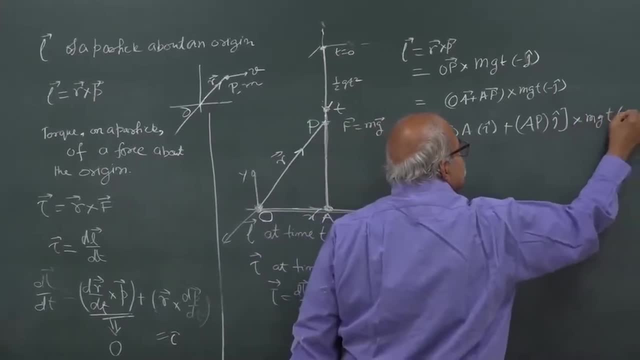 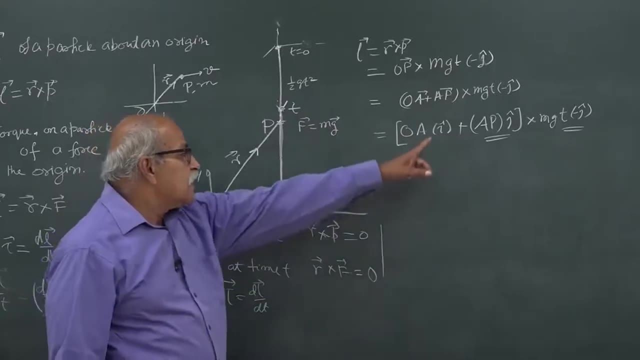 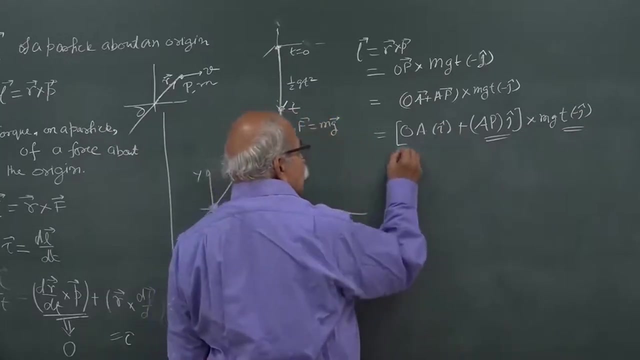 And cross mgt. So this i is only oa times u, and this is u fiz, this is u fiz. So this is oa through oa divided by mgt minus j cap Ugh, Or is it j open? Whoops, I forgot to add one. so uit is open because it is open, because k is not z it's. 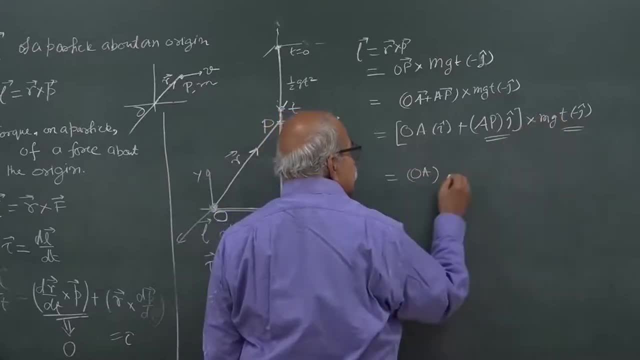 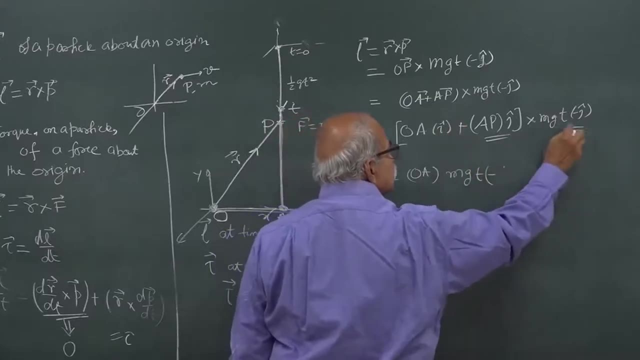 just ui. The lag is for jcab. So for jcab cross jcab is 0.. But i cap cross jcap is not 0.. It is k cap. So this is oa multiplied by mgt and then minus, and i cap cross j cap is k cap. 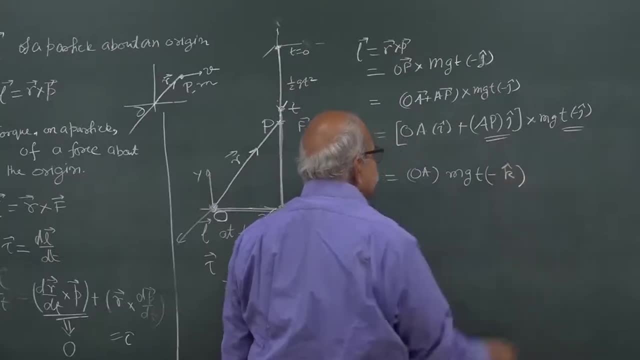 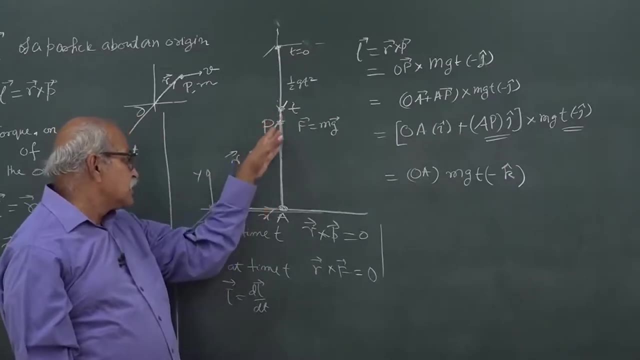 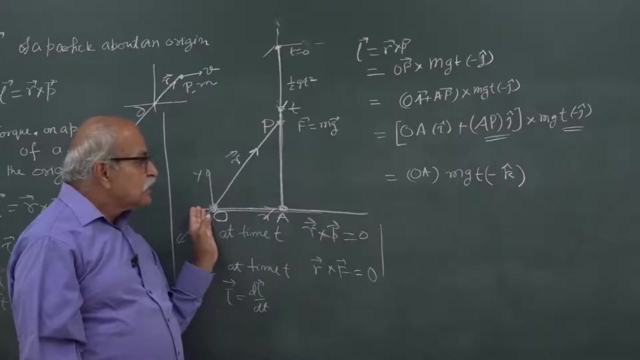 So there is some use of this mistery. We've got mgt, k cap, OA is fixed. the particle falls like this: So all the time OA is fixed. So OA has a magnitude, depends where we have chosen the origin and then m, g, t in minus k cap direction. 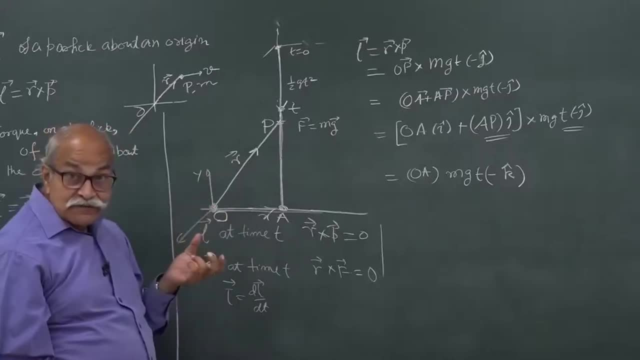 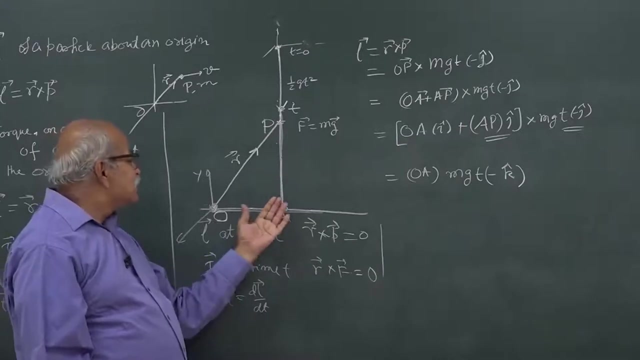 and k cap, remember, is now perpendicular to the blackboard, So the particle is falling along this, parallel to this y axis. This particle is falling parallel to the y axis, but its angular momentum is in z direction, negative z direction. If this is x, this is: 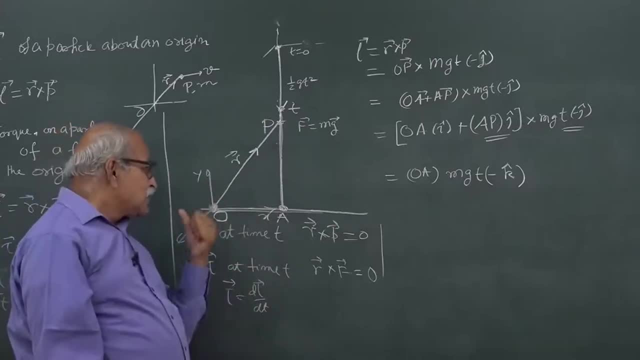 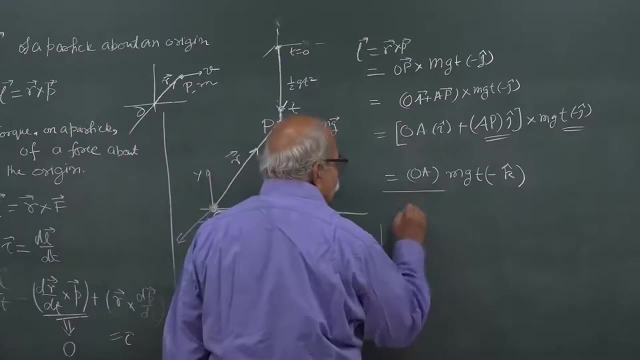 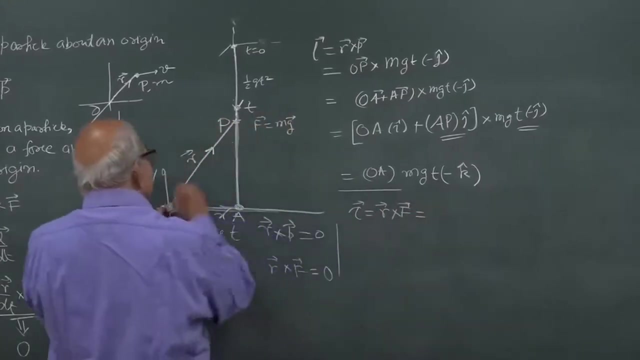 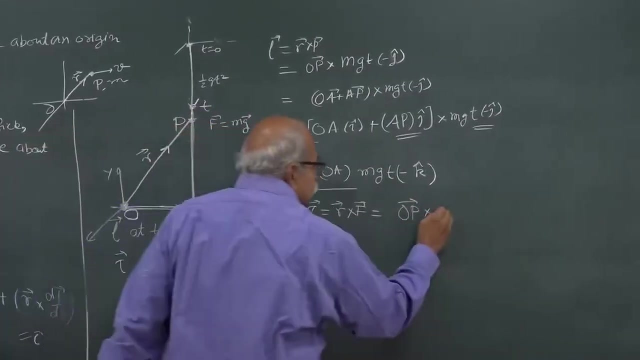 y z is coming towards us and minus k cap means it is going into the board. So that is L. What is torque? What is torque? Torque is R cross F And R is OP vector, So OP cross F. F is m g in the downward direction, So m g times. 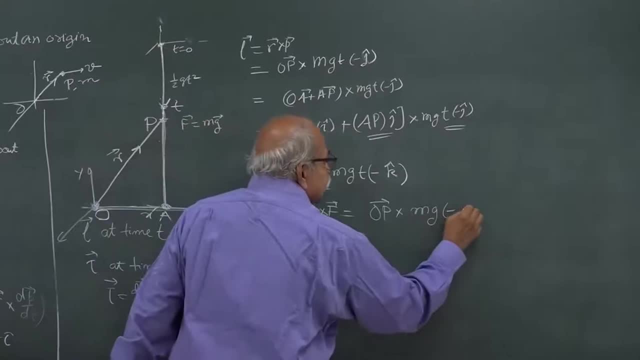 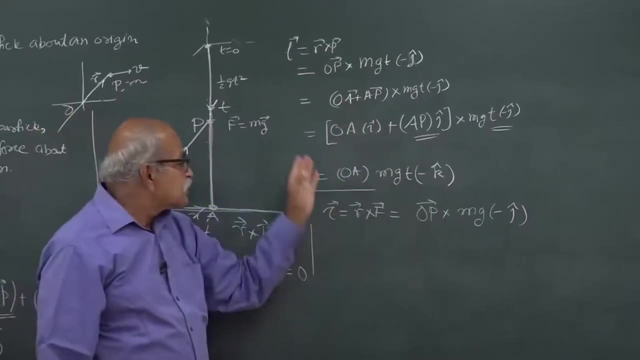 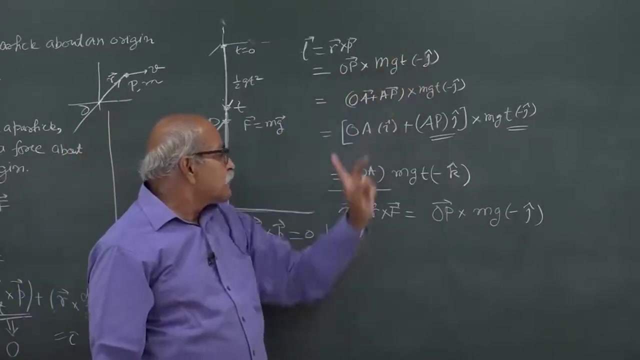 minus j cap. So minus j cap. Look at this expression for L and this expression for torque. What is the difference? OP cross m g, t minus j cap. OP cross m g minus j cap. Only this t is not there, otherwise everything is there. So now, 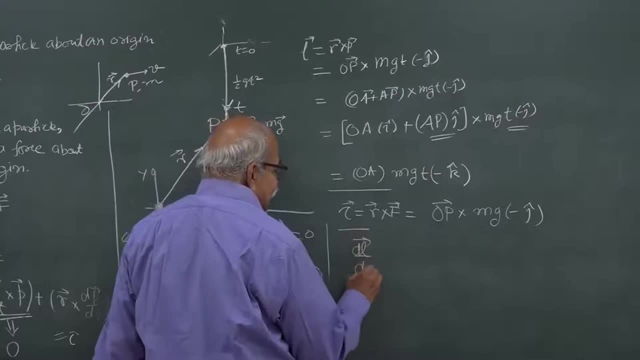 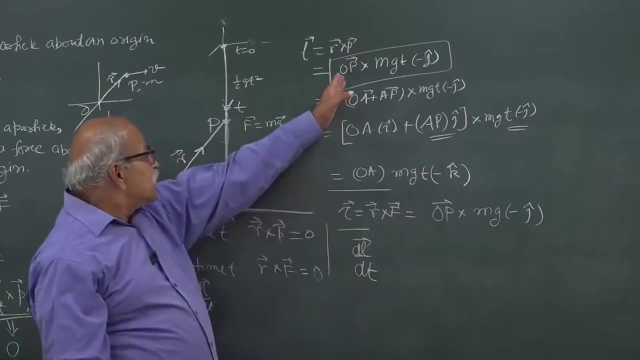 if you do this, d L d t, Here is d, L, This is d, Here is L, This is L, And I am doing d L d t. Differentiate this with respect to time. OP is a fixed vector. No, OP is not. 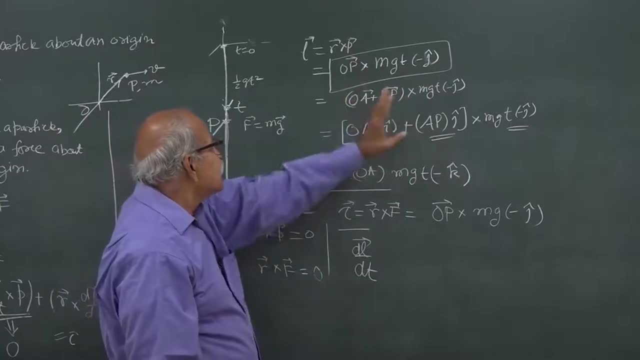 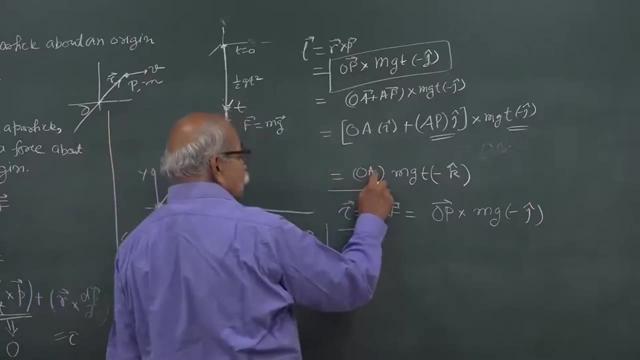 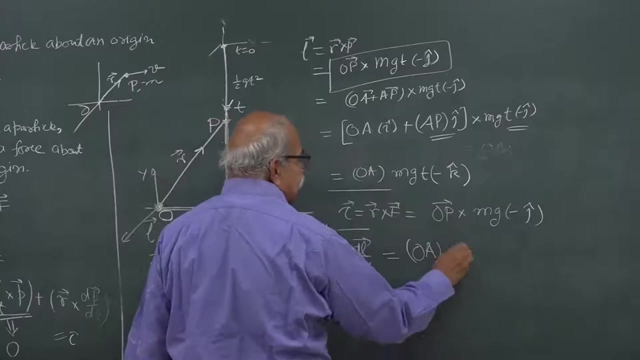 fixed vector OA plus AP. You can write it like that, So your Your d L, d t. if you take from here: OA is fixed, Correct, OA is fixed. So this is OA, And then m g is fixed And differentiate with respect to time, So it is 1.. So it. 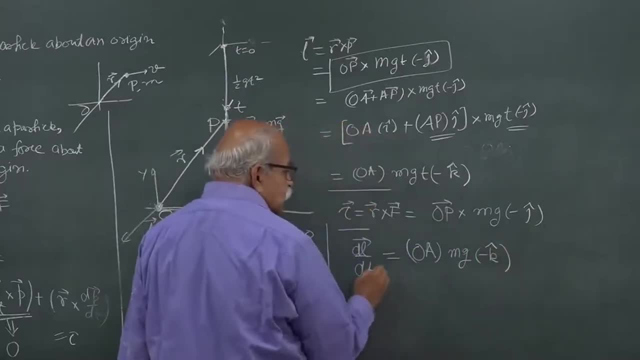 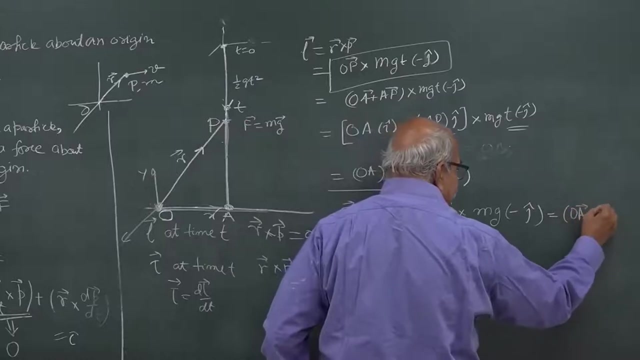 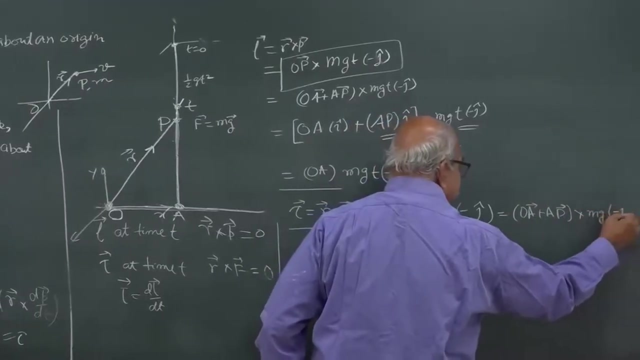 is minus k cap, So OA into m g And then differentiated here minus k cap. And what is this? That also you can work out: This is OA plus AP And then cross m g and minus j cap and 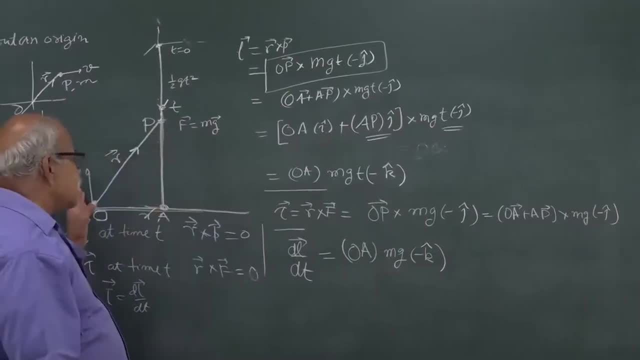 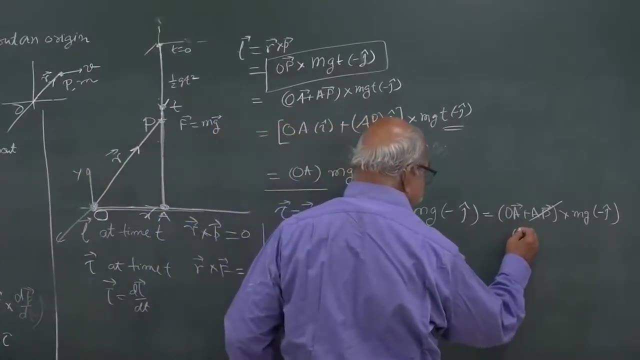 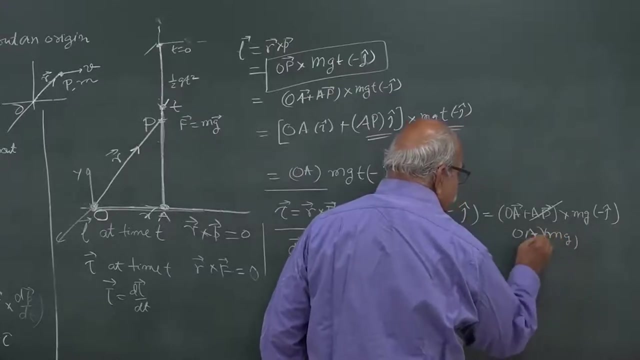 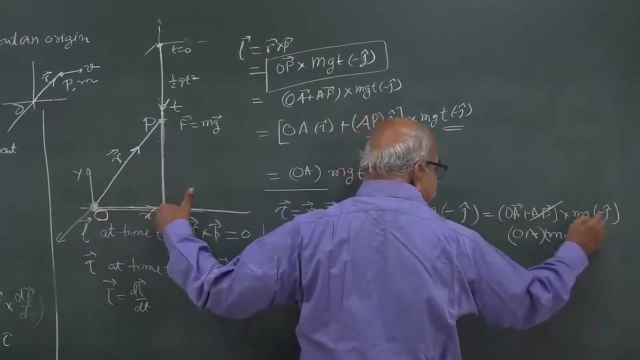 once again, AP is parallel to this y axis, So this is part will go away And what you will have is this OA and then m g here, m into g here, OK, OK, Ok, OK, OK, OA here. and this OA is in x direction. so x i cap and j cap is k cap. so minus k cap, simple. 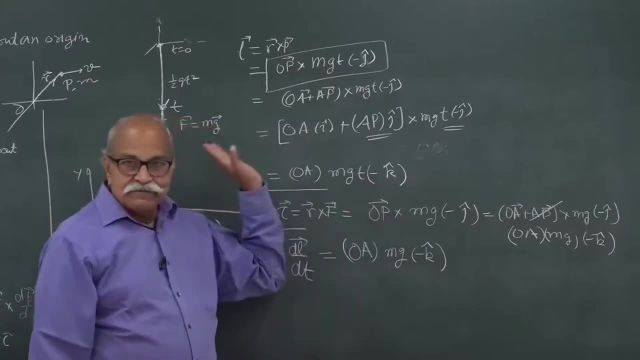 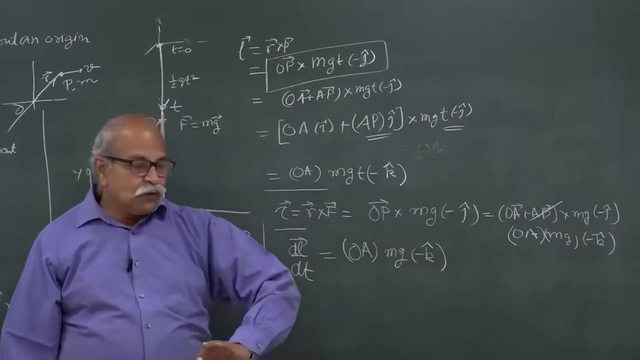 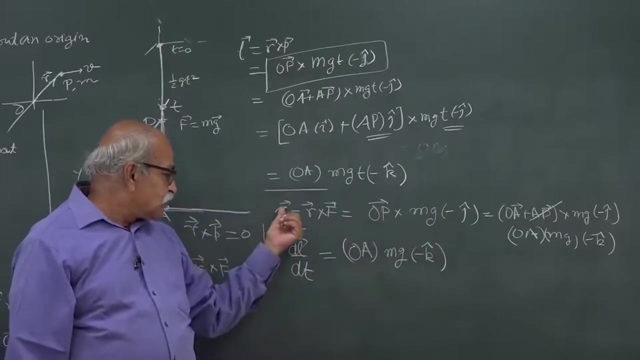 Same as this torque is same as this dldt. so even for a particle which is falling vertically under gravity, if the origin is chosen in a certain way, you do have angular momentum, you do have torque, and then the rate of change of angular momentum is equal to torque. that 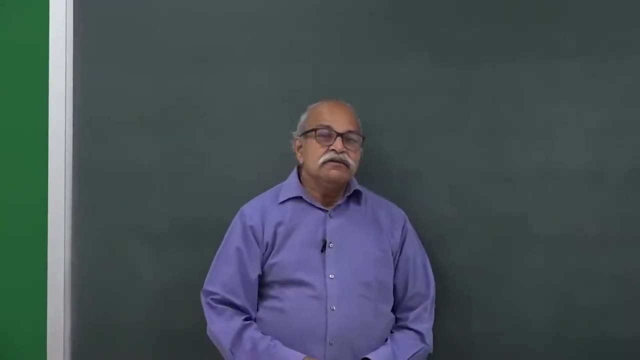 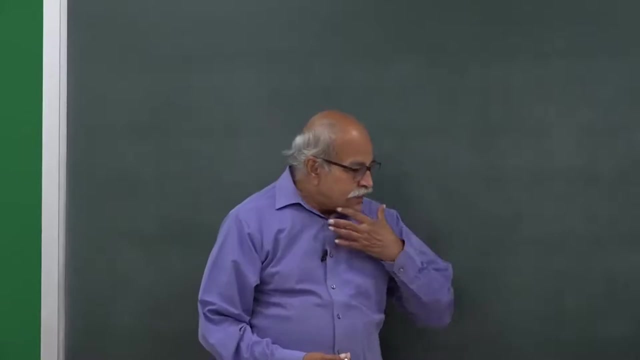 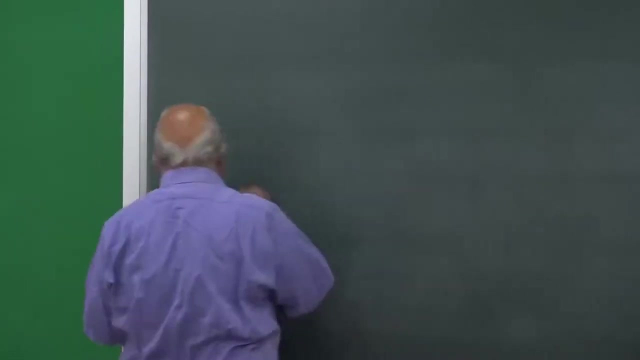 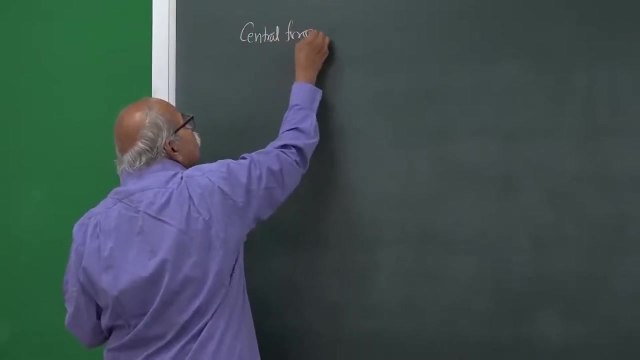 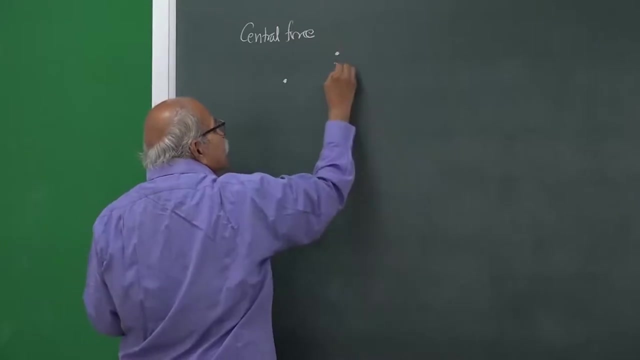 equation is valid. So my next example is from central forces, and we will be talking at length about the central forces here to introduce this idea of angular momentum and its use. So we call it central force Because you have a force center, so you have a point and the particle is can be anywhere. 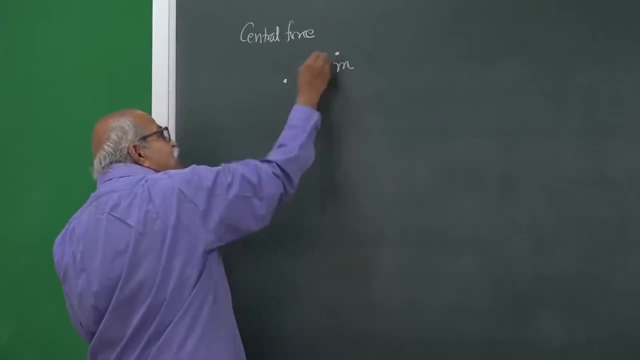 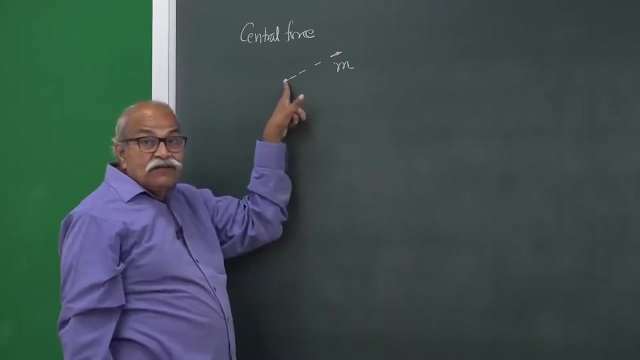 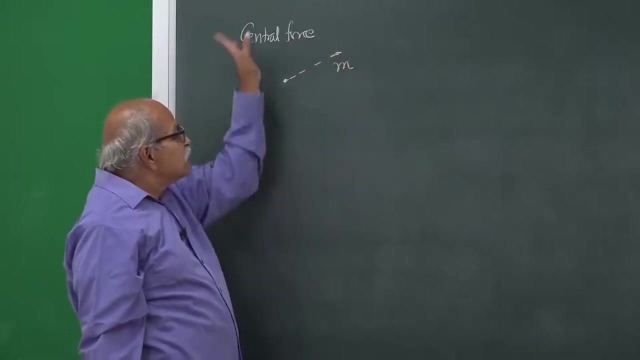 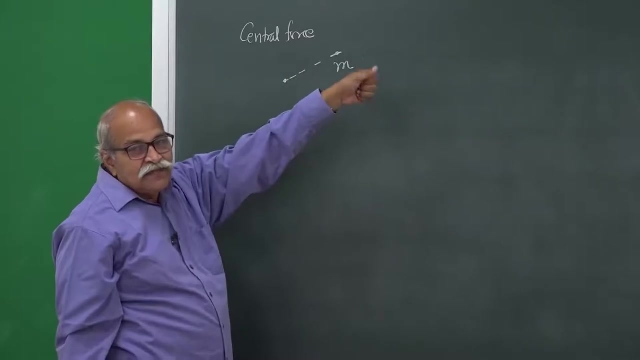 and then the force on the particle is always along the line joining the particle from this fixed point that we call force center or center of force. So you have a fixed point. the particle can go anywhere in the whole space, but wherever it is. So if you join the origin with that position of the particle, the force on the particle, 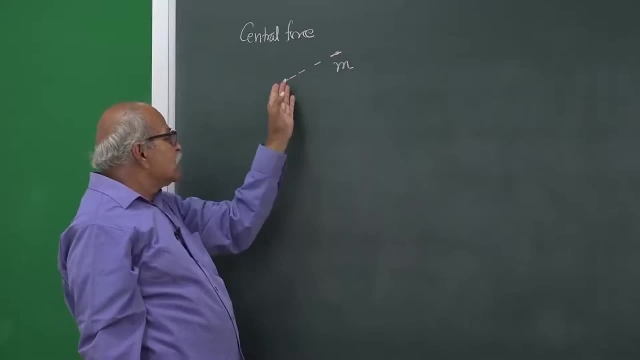 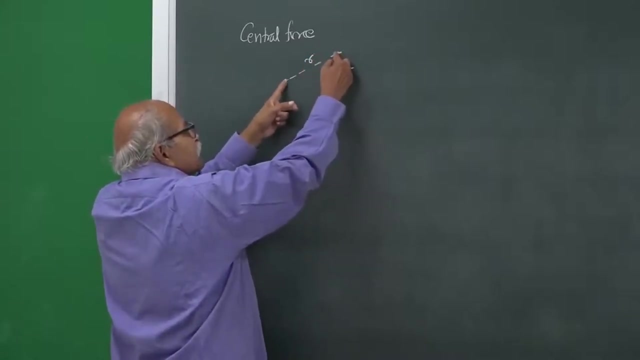 will be along that line, either towards the center or away from the center, and then the magnitude of the force depends only on this distance from this fixed point. if that happens, we call that force as a central force. so I can write for central force: f at r is equal. 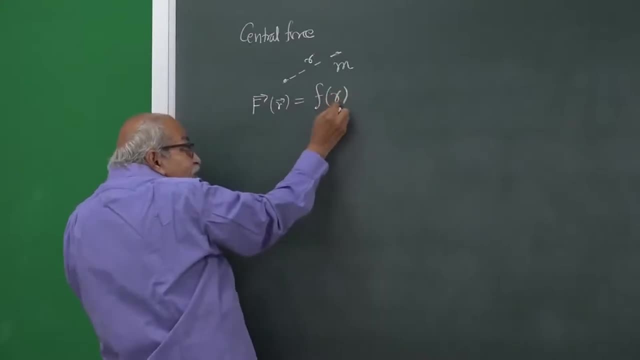 to some function of r, R without vector. here r is which vector, here r is without vector. and then r cap. what is r cap? just tell. first let us see what is this r vector and what is this r? R vector is, as usual, position vector of the particle at time t. 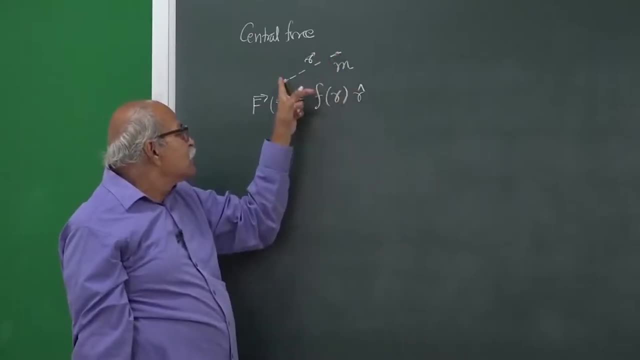 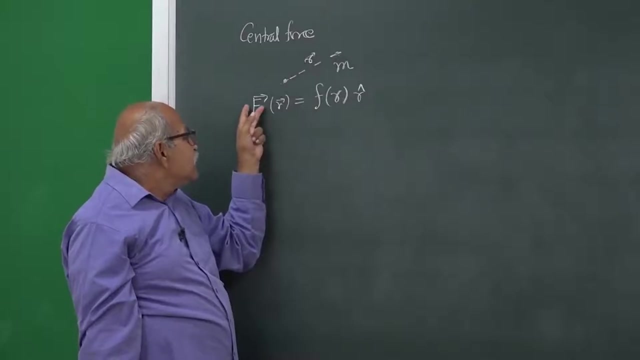 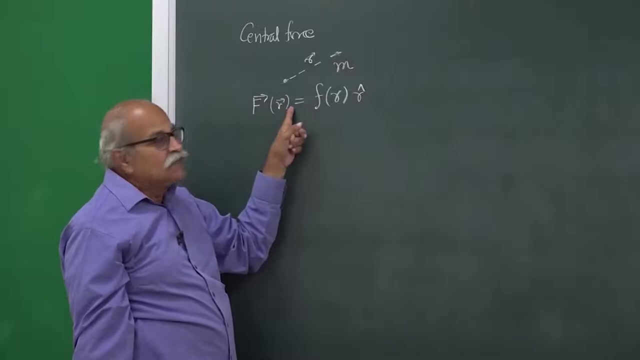 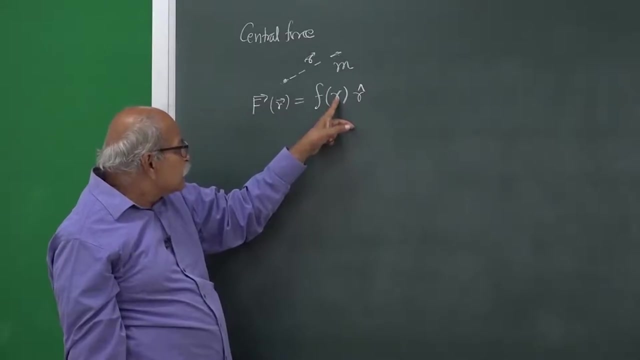 So at time t the particle is somewhere and I join the origin and the particle and that vector is this r vector. 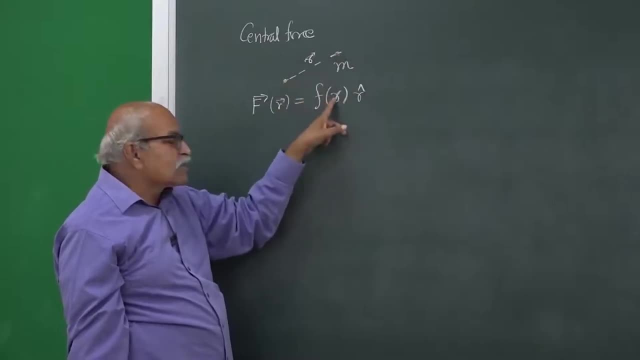 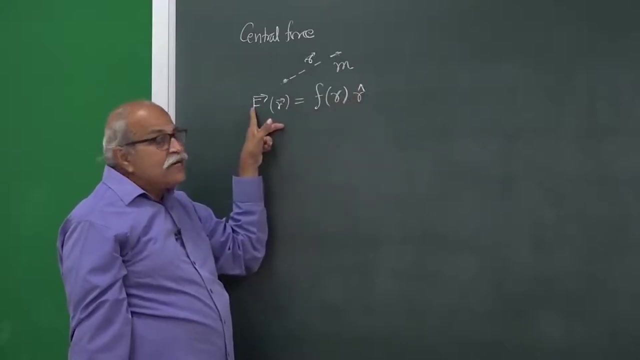 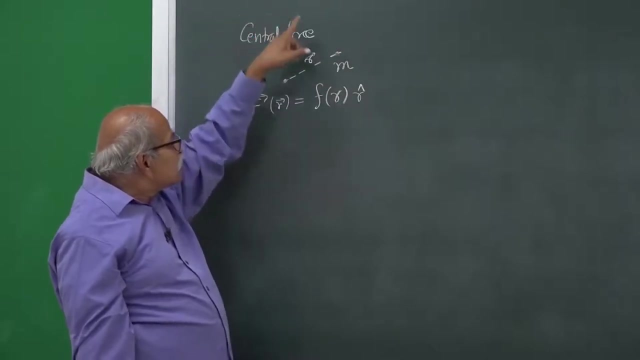 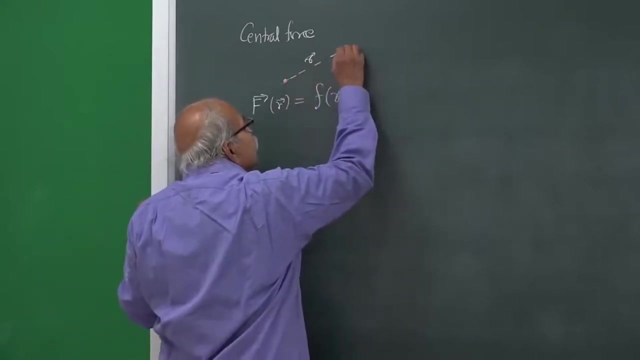 direction is the direction of the force. It need not be in general, it need not be in this direction, but for a central force it has to be in this direction. This r cap vector is along this line and in the increasing r direction unit vector along the direction. 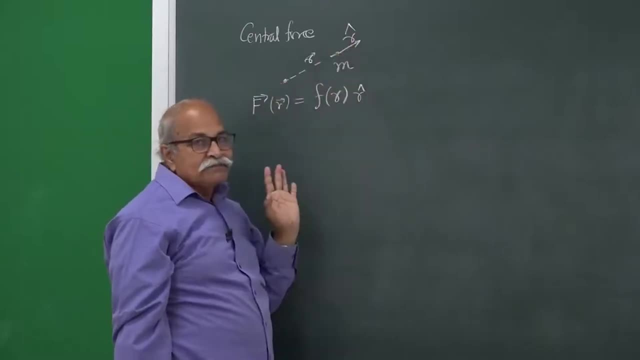 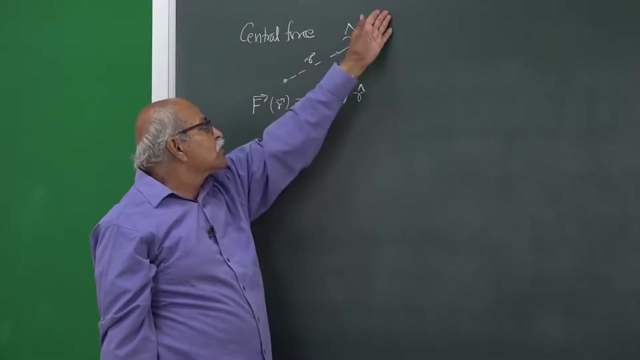 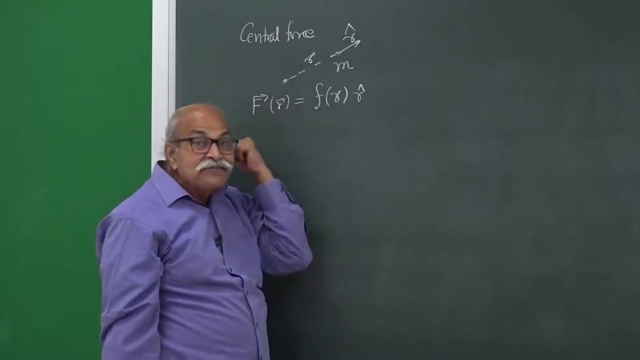 of this position vector. this is known as r? cap. So this f? r, if it is positive, then the force is away from the center of force. If this f? r is negative, then the force is towards the center, attractive or repulsive. 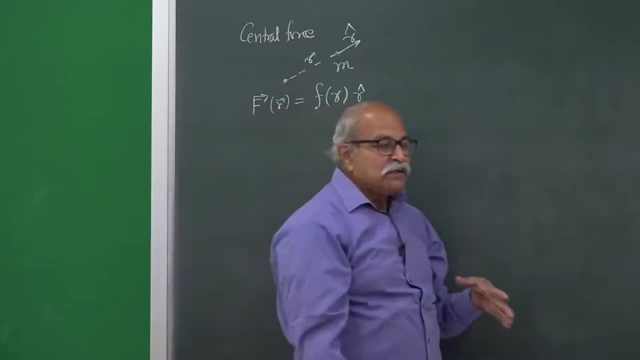 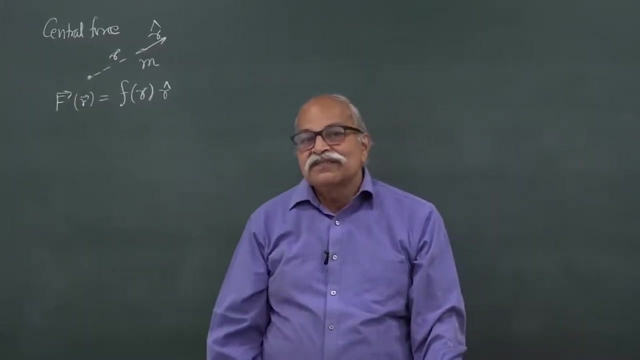 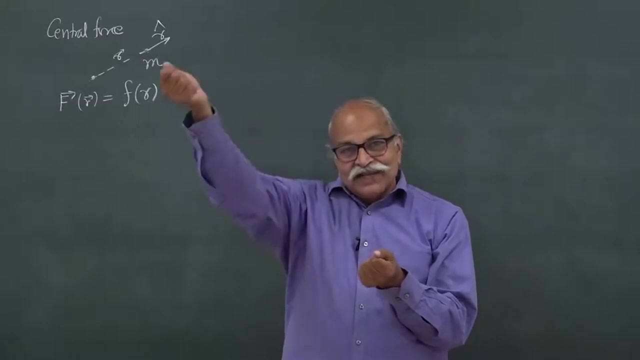 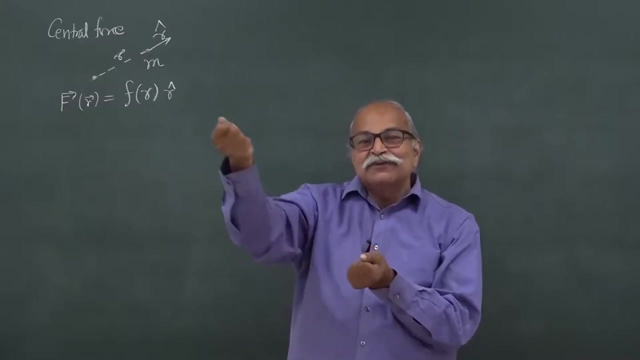 So we have enough examples for such central forces, at least approximately our planetary system. So we have the Sun and the planets. So Sun attracts the particle, the planet, wherever it is. So the force is in the direction of that Sun. that means opposite to the position. 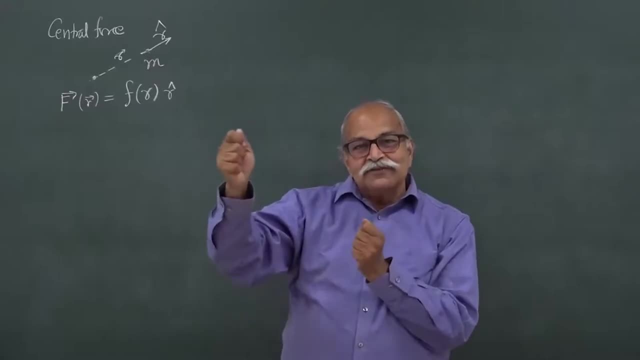 vector and the magnitude depends only on the distance between the Sun and the planet. The Sun is given, the planet is given. so m 1, m 2 is there. capital G is there, so it is only by r square. It depends only on the distance between the Sun and the planet. The Sun is given, the 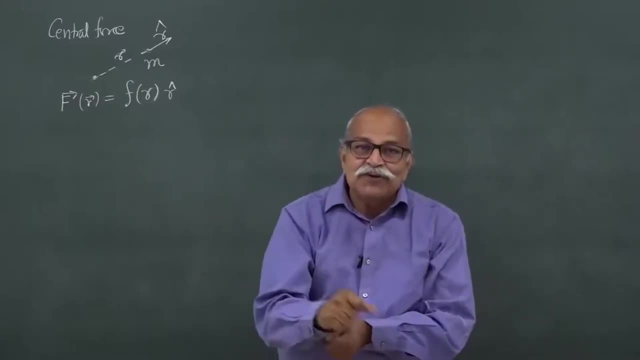 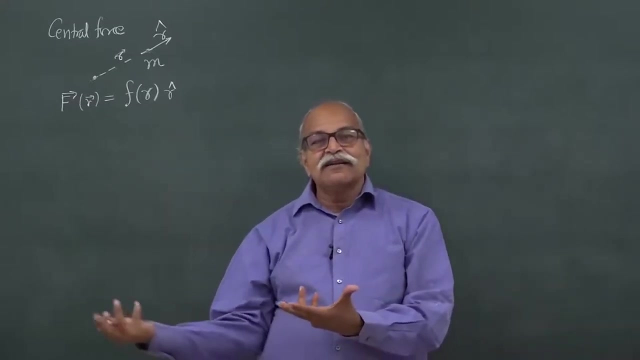 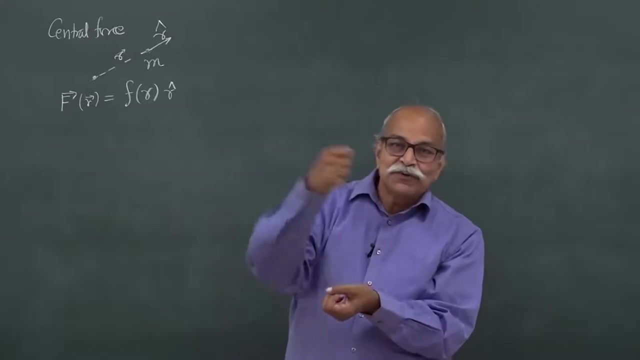 force is only on r, not on the direction, not on the direction. So, or let us say Bohr's model of atom: you have a proton and you have an electron, and then in that model the electron is supposed to go in some circular path. So all the time. 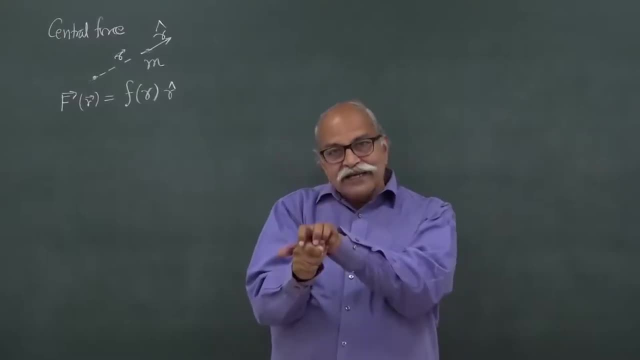 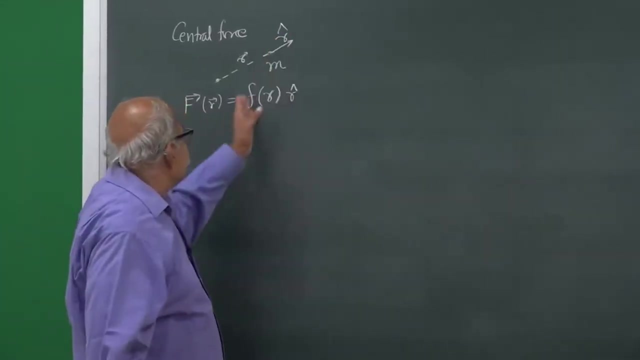 the force on the electron is towards that proton which is taken as origin, and the force on the distance only q 1, q 2 by 4 pi, epsilon naught r square. So you have so many examples, So let us try to study this Now. suppose this particle is acted upon by this central. 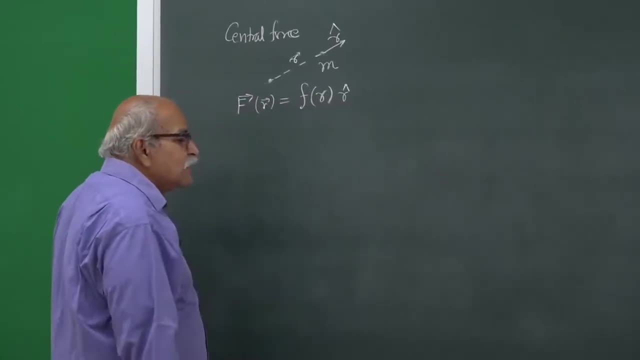 force, and we ask: what is the angular momentum of the particle? how do I write the angular momentum of the particle? So first let us take some axis And in this process I will be telling you more about another coordinate system in two dimensions. 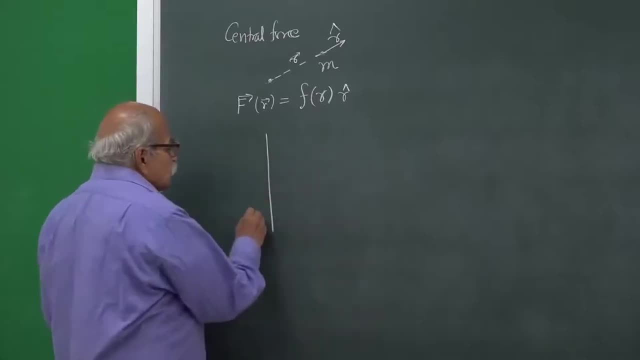 which is known as plane polar coordinates. So I have x axis and y axis and then the particle is somewhere. and if I join the position of particle from the origin, this vector is the position vector r and the unit vector along this. So this position vector is known as r, cap, and then this angle I can call theta. and if 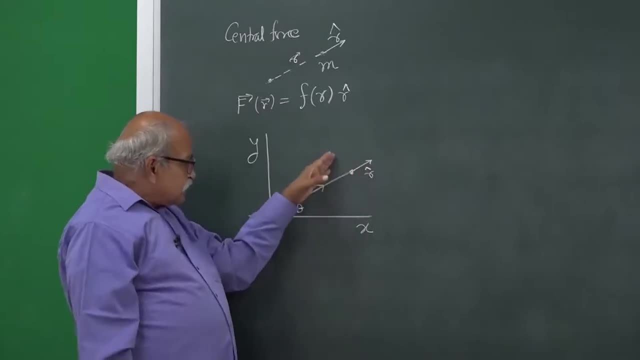 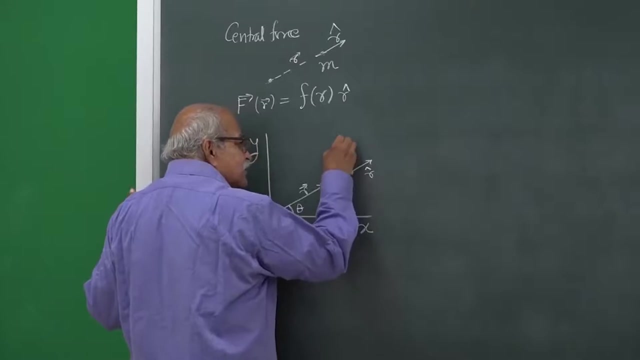 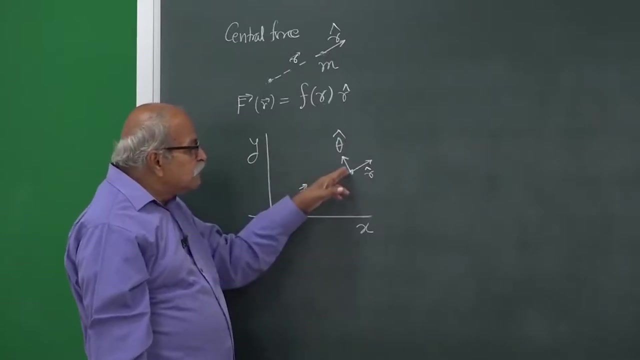 you do not increase the distance but turn it so that this theta increases. So the direction in which r is not changing but theta is increasing. that means perpendicular to this. this direction is known as theta cap. So if I take the particle in this direction, this theta will increase, If I take it infinitesimally. 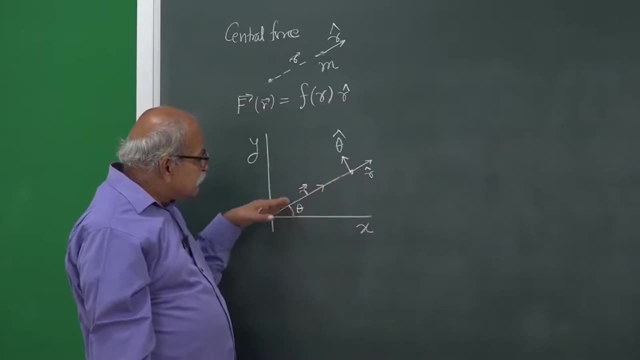 small distance. here. this theta will become theta plus d theta, But r will remain the same same means. if it is infinitesimally small, there is no component of that displacement in the r direction and therefore for that infinitesimally small displacement we will 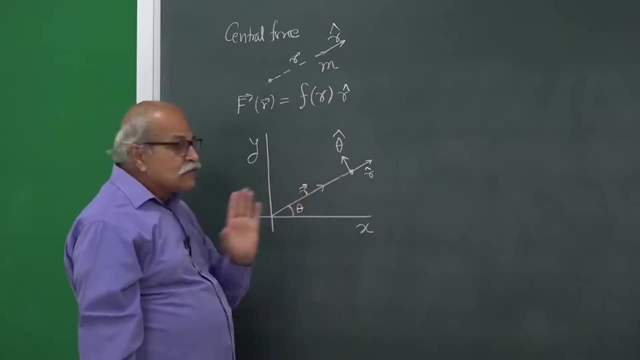 take that r is constant, only theta is changing. So what we are doing in this case is that we have r is constant, this is r cap, this is theta cap. and if I drop a perpendicular here, this is x and this is y to get the position. I can write what is x and what is y. I can also write what: 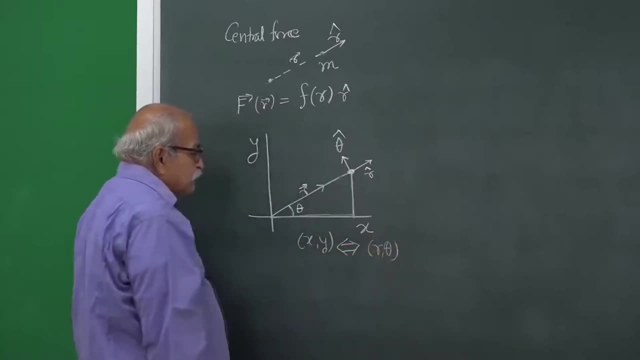 is r and what is theta? If someone says that, all right, it is at a distance of r from the origin and this line makes angle theta with the x axis. that also tells me that the particle is here, provided the particle remains in this x y plane. If it is in the x y plane, yes, give. 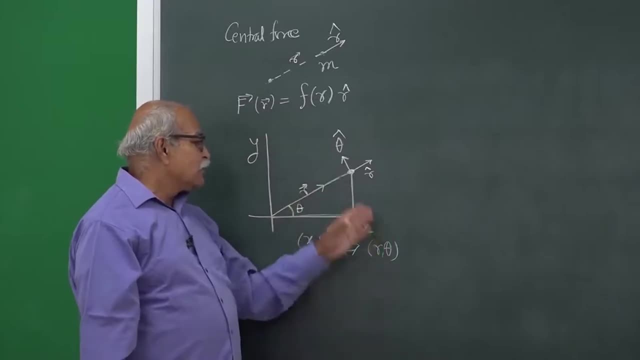 me r, give me theta. I know that it is in this plane and I know where the particle is. If I know that it is in x y plane, give me x, give me y. I know that it is in this plane and here is x, here is y. 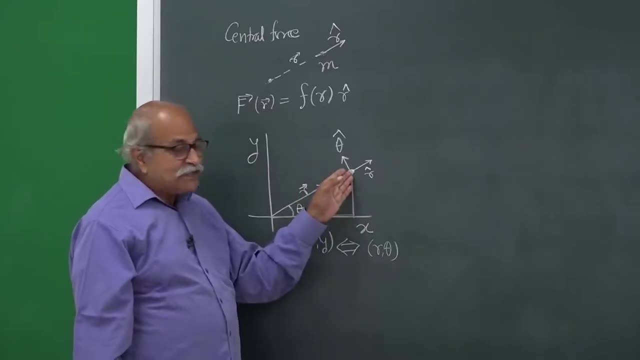 And this should be the particle. but if it is, it is leaving this x, y plane and it moves in a space, three dimensional space. z is also there. then neither this is sufficient nor that is sufficient. Let us come back to our angular momentum. So, angular momentum. 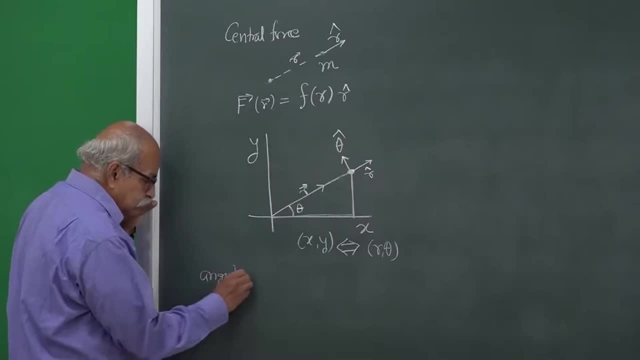 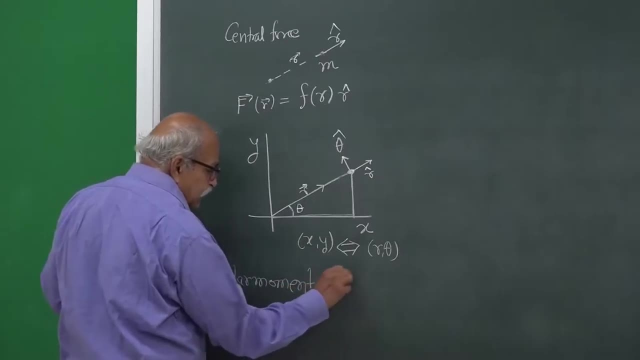 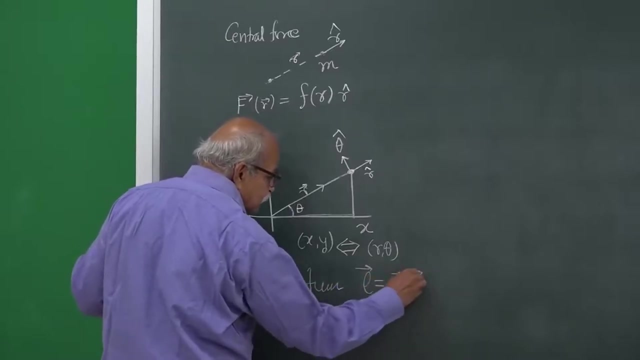 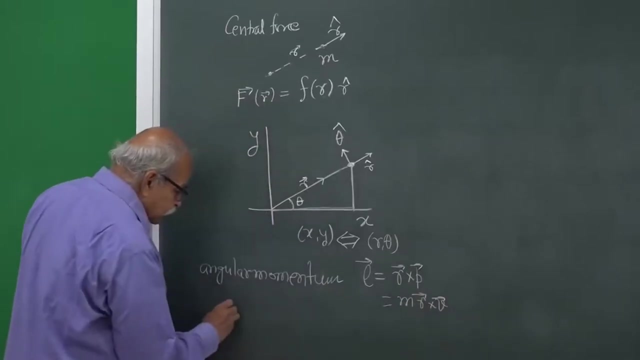 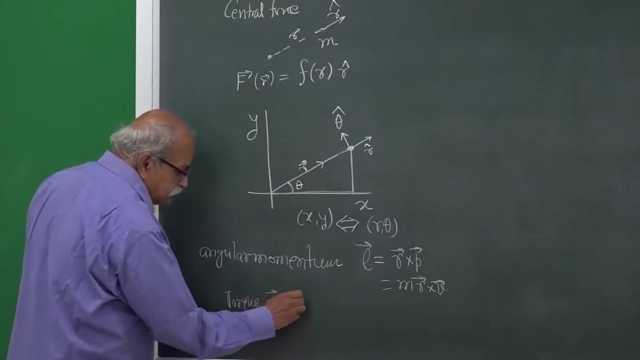 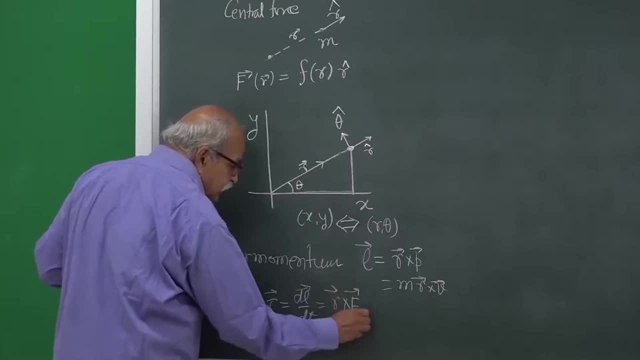 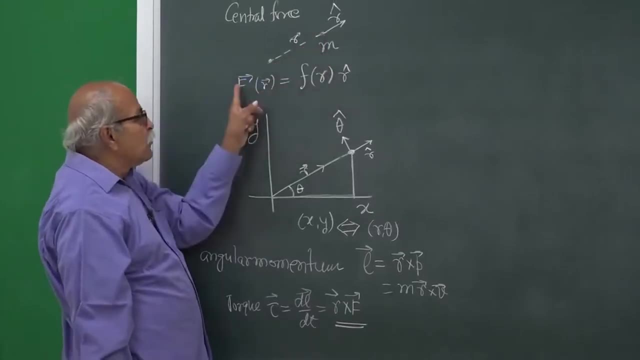 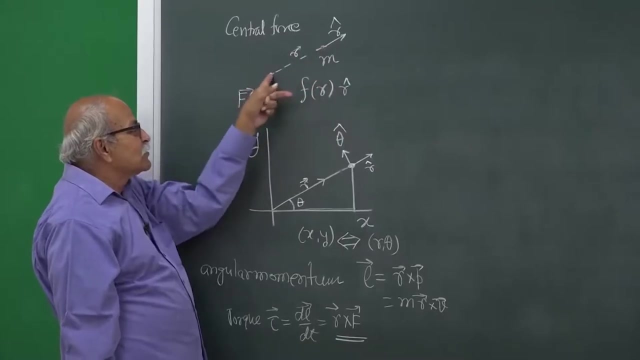 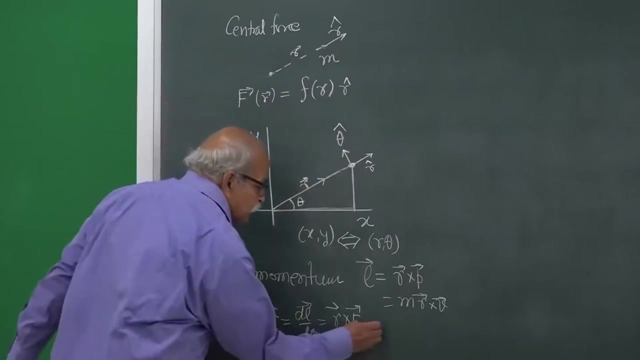 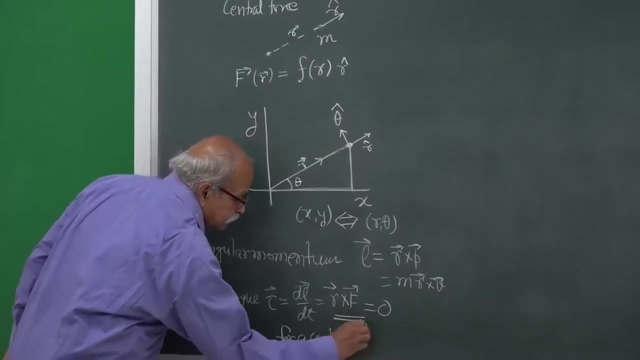 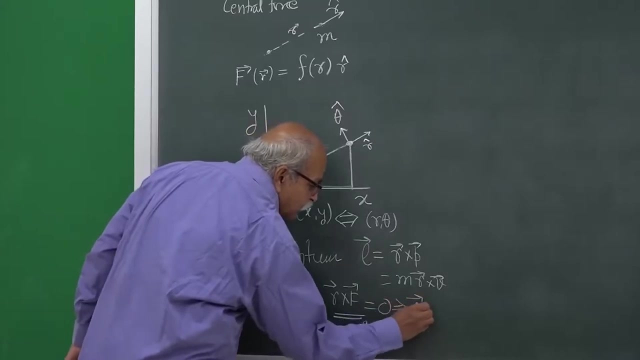 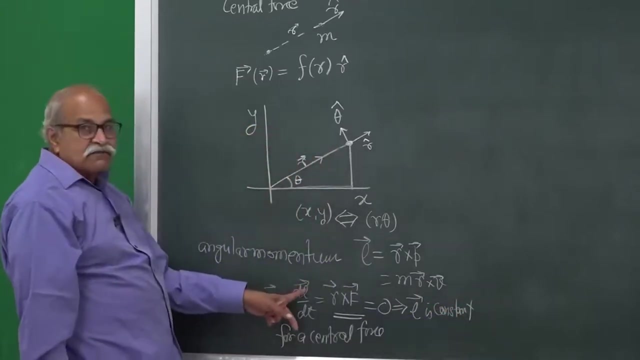 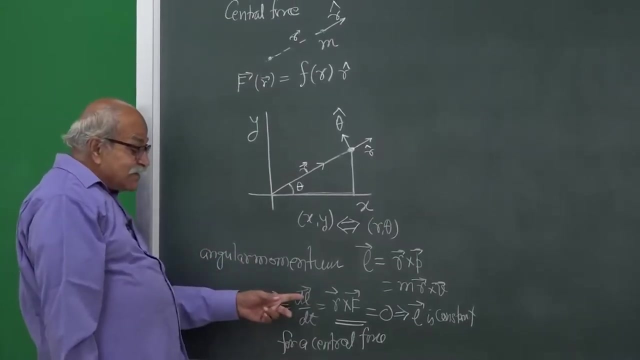 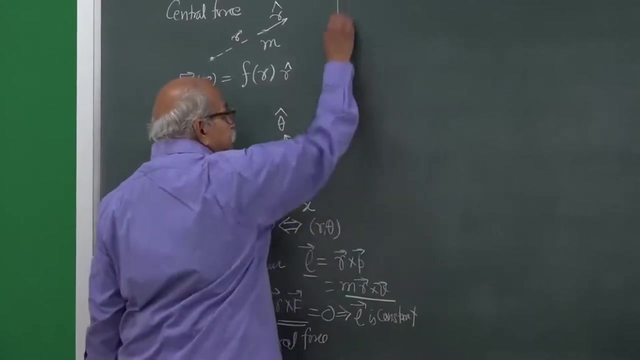 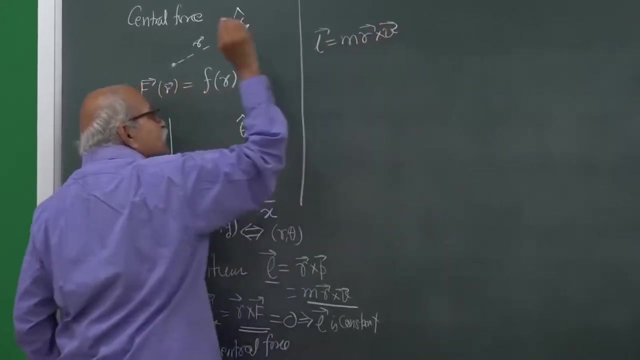 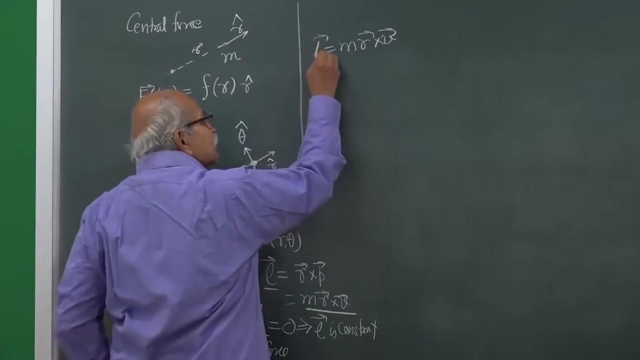 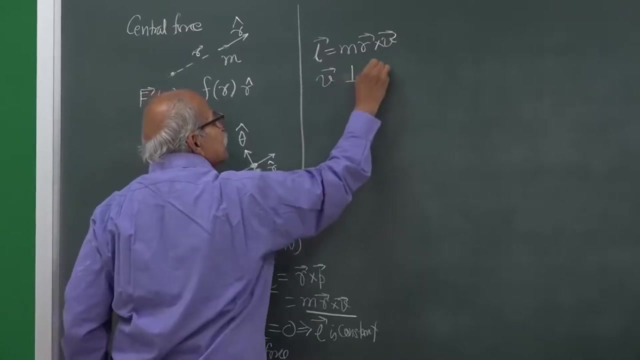 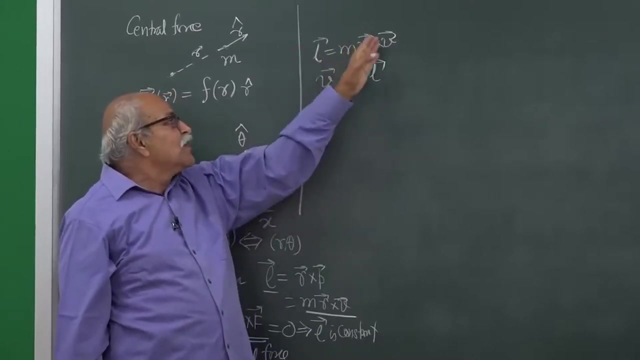 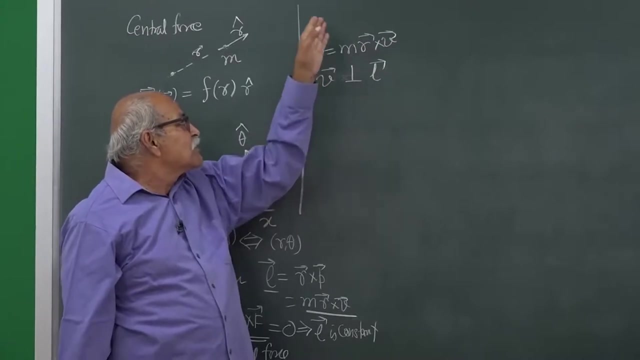 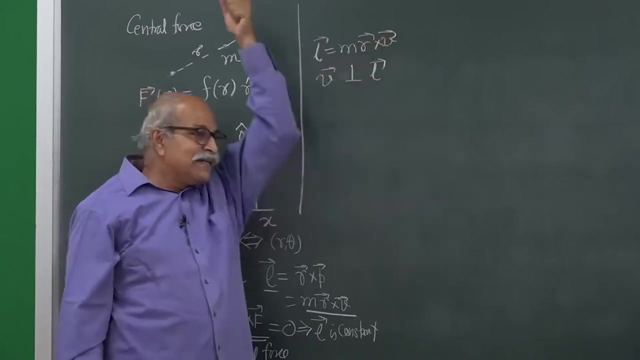 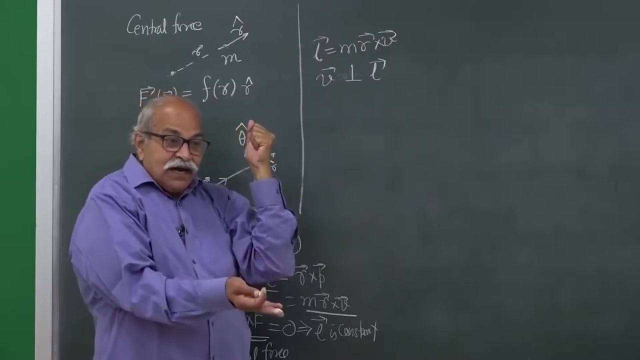 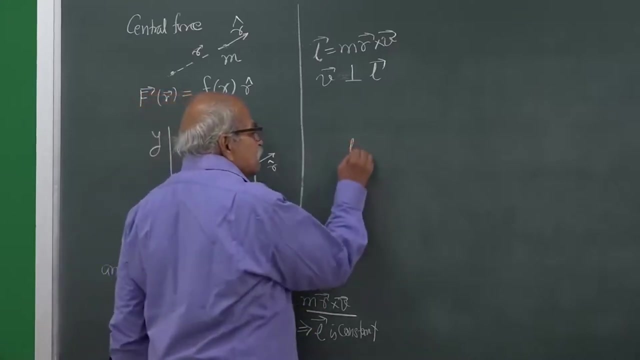 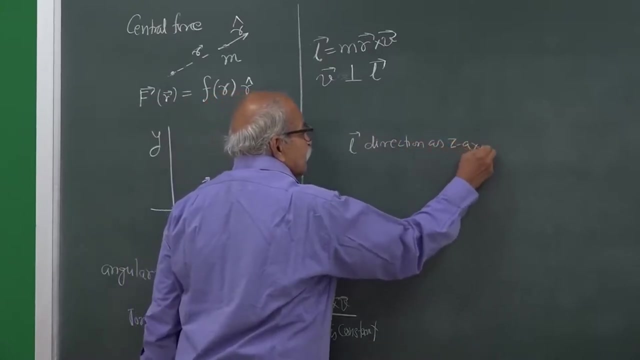 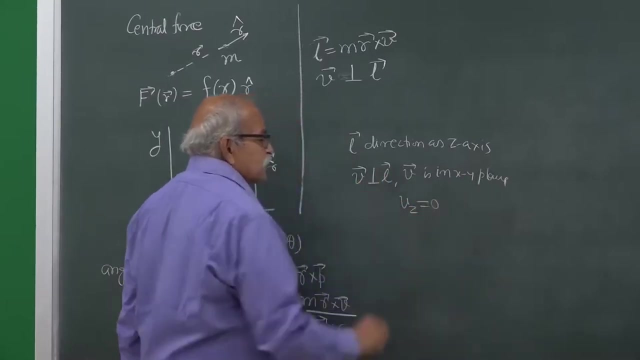 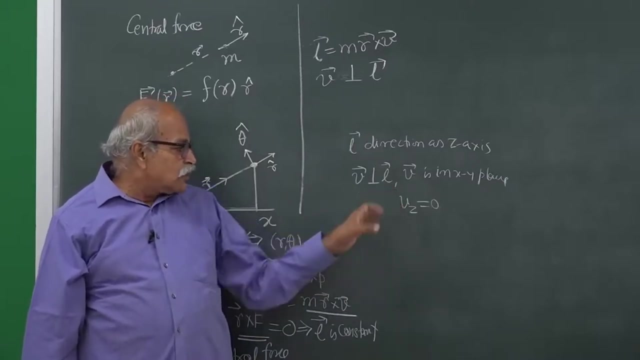 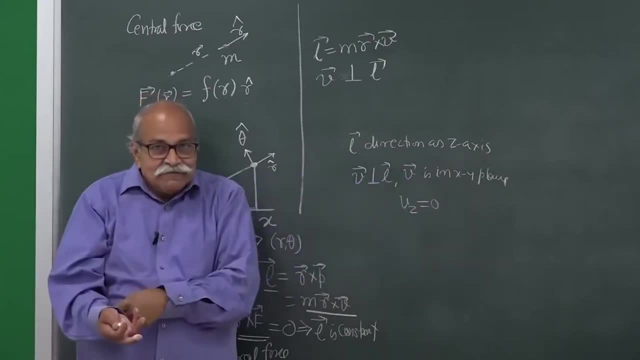 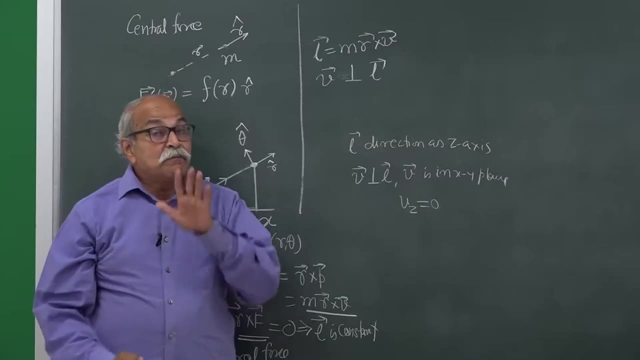 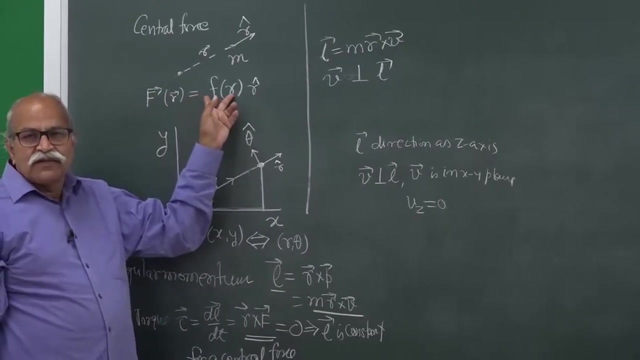 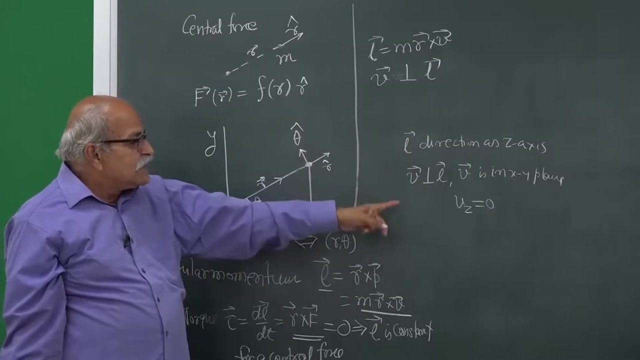 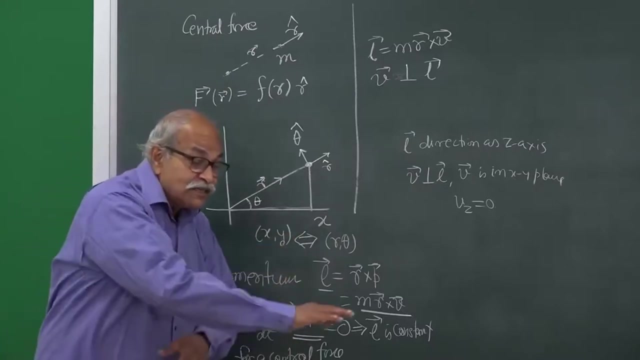 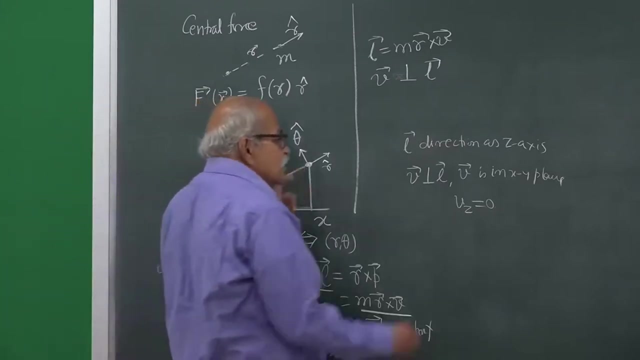 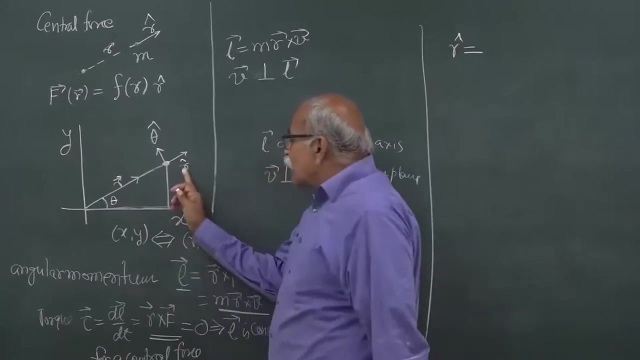 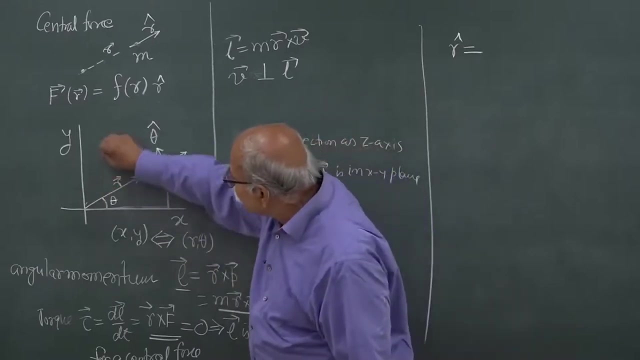 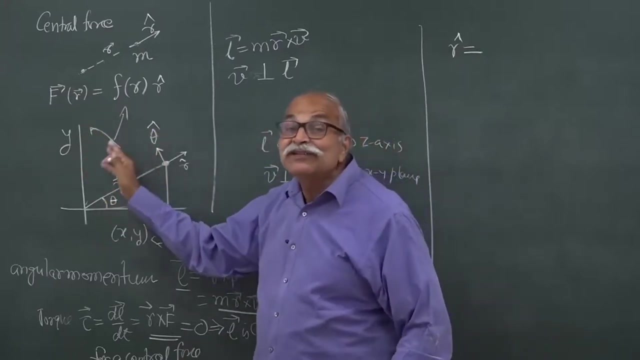 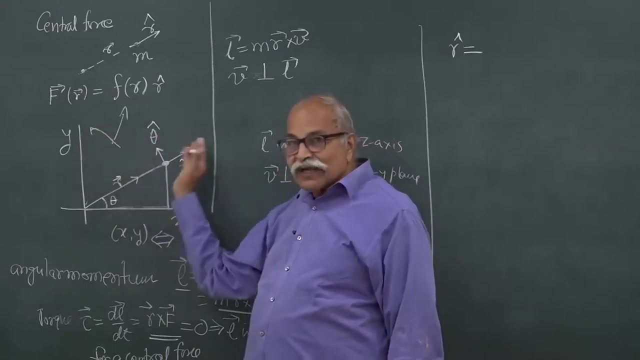 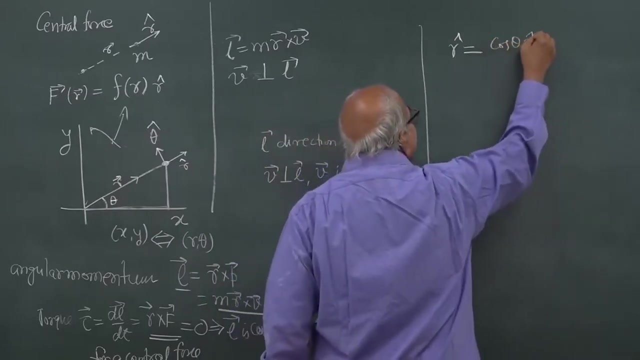 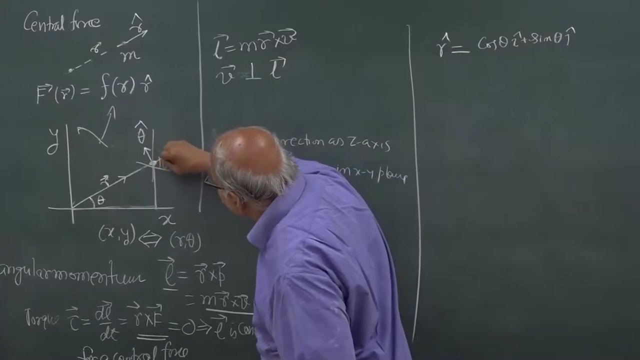 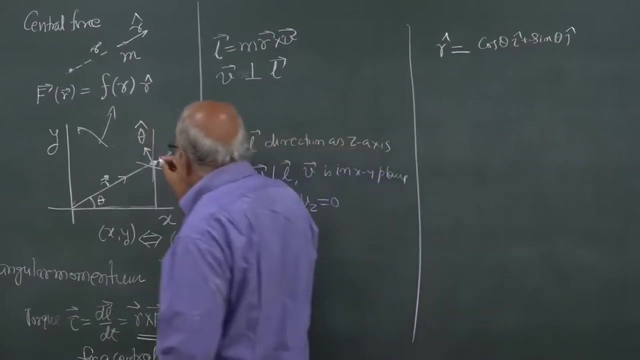 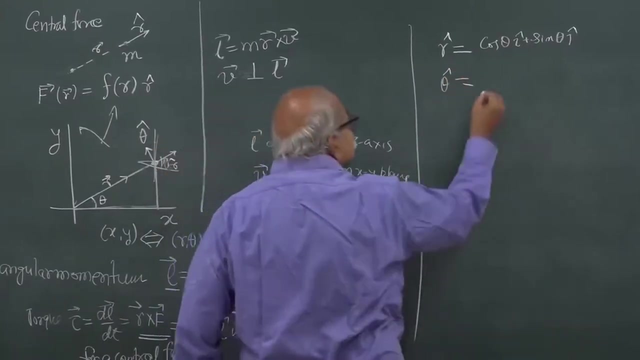 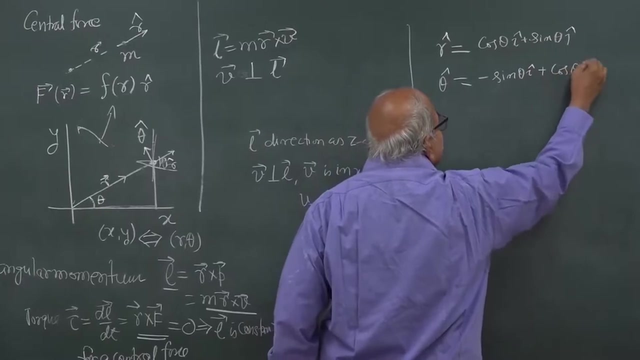 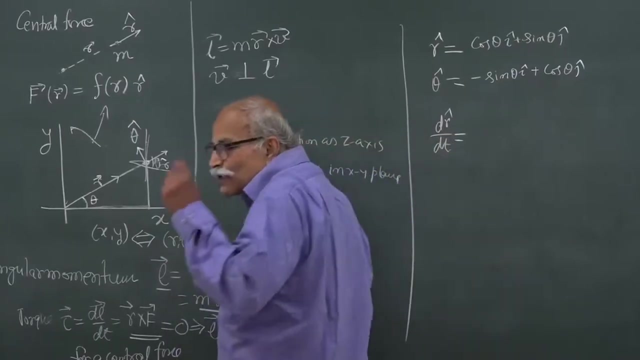 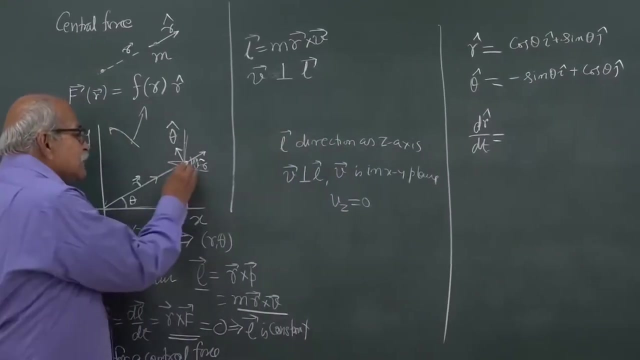 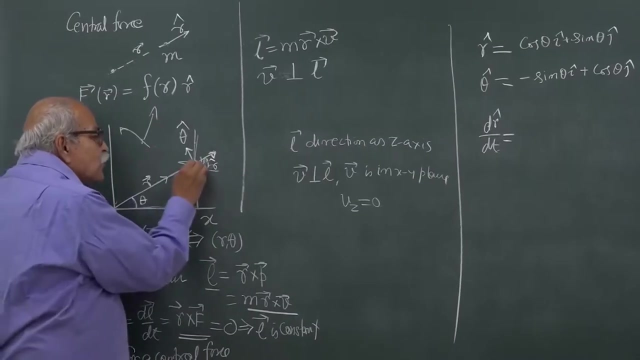 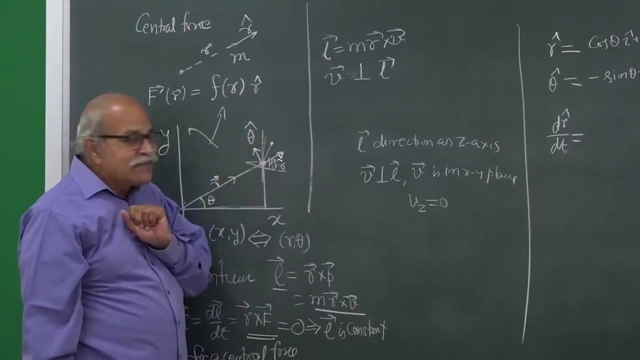 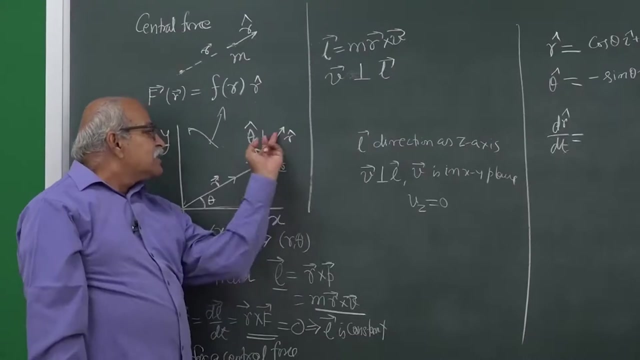 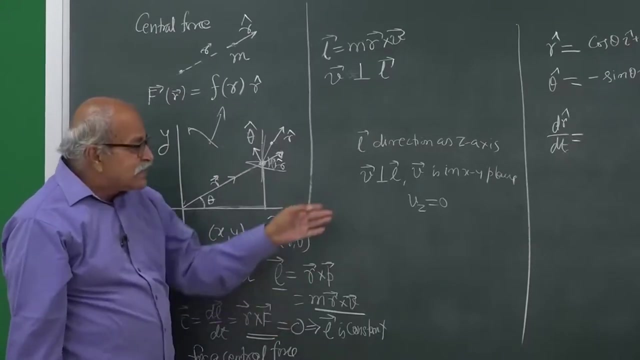 minus that vector, that is change in r cap, and therefore I divide by d t and I get this. 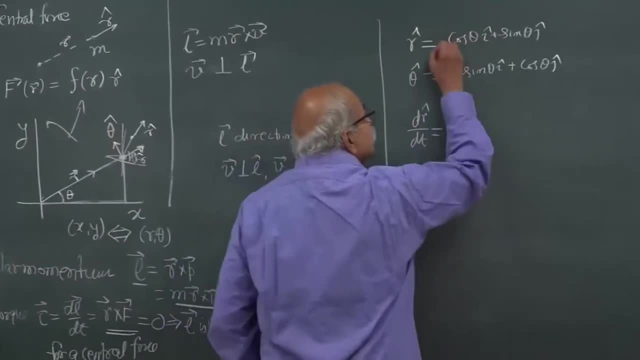 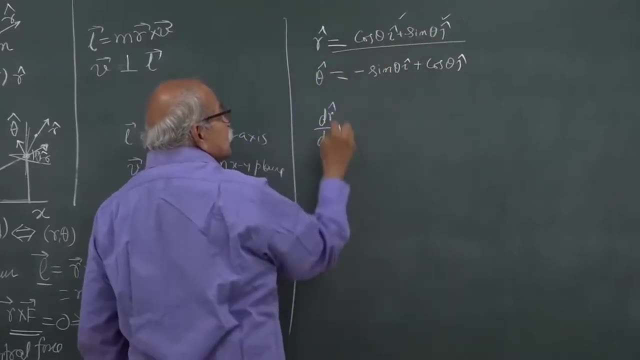 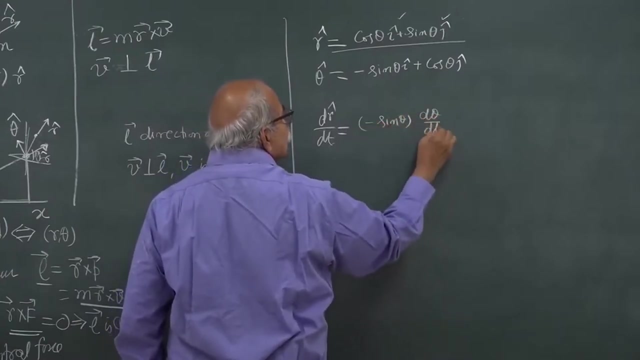 d r d t. So here is r. these are fixed vectors. i cap, j cap. theta can vary. theta is variable. theta can change as the particle moves. So this is minus sin theta and then d theta d t and plus cos theta and then d theta d t. here is j cap, here is i cap and this is minus. 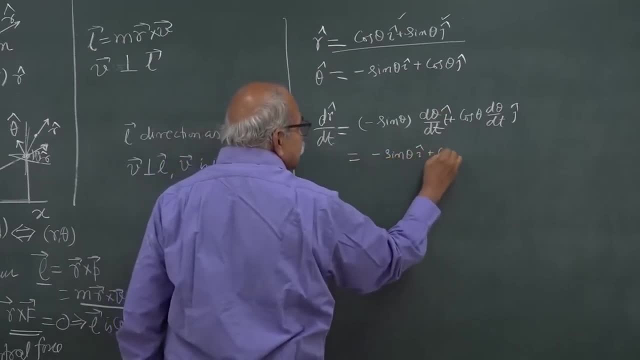 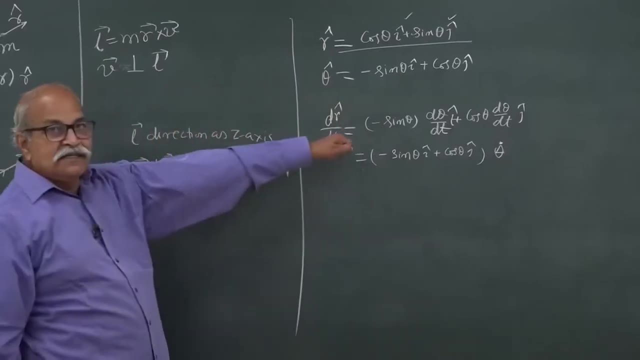 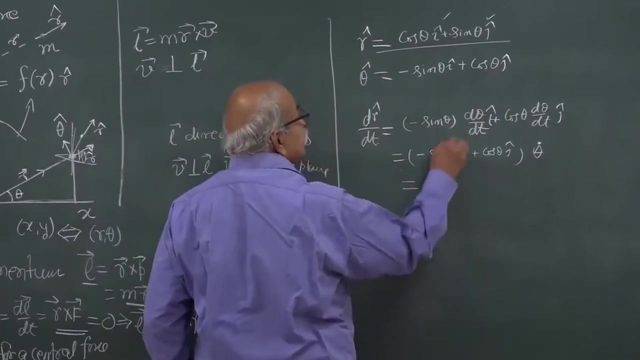 sin theta i cap, plus cos theta j cap and theta dot. and when I write dot, it is d d t, d d t of theta, And this is theta k, This is theta cap, theta dot, it is theta dot, theta cap. So d? r cap d t is theta dot, and 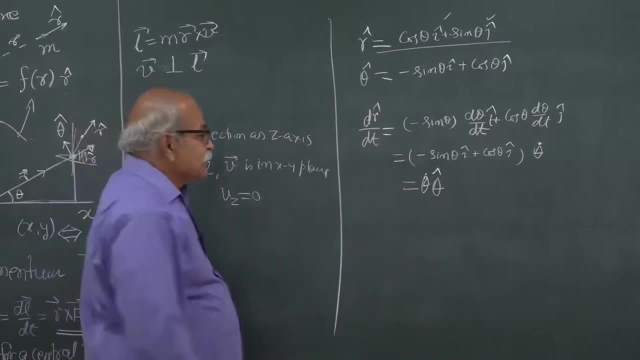 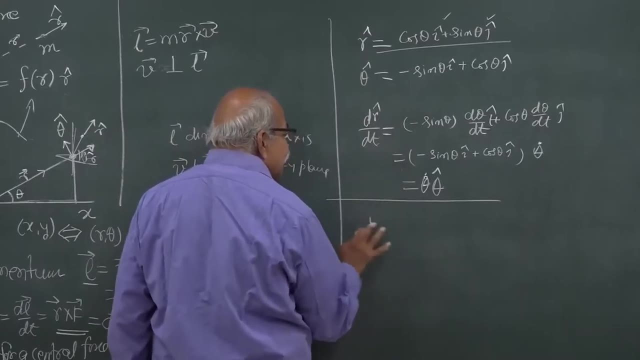 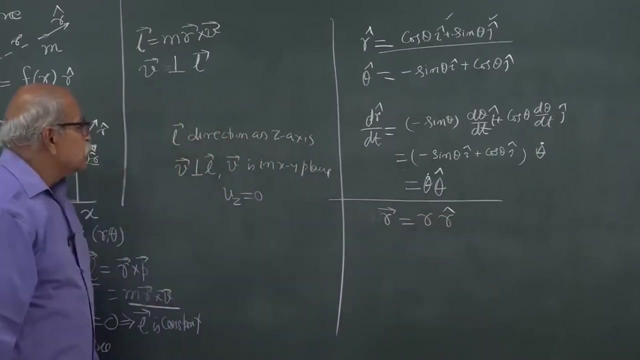 then theta cap. So once again, let us write this: l vector, you can write what is v vector. what is first r vector? r vector is r, r cap. can you see this? can you see this? r vector is r, that is the magnitude and the direction is r cap. So r vector is this magnitude, r. 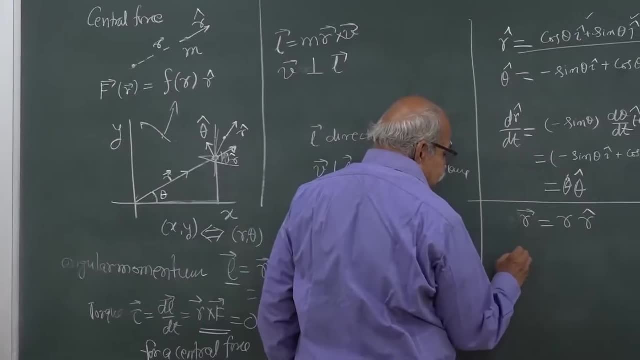 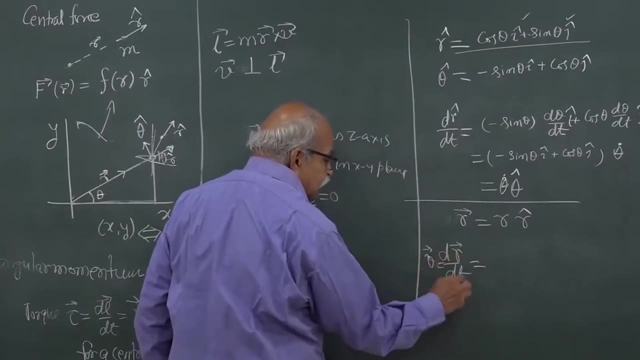 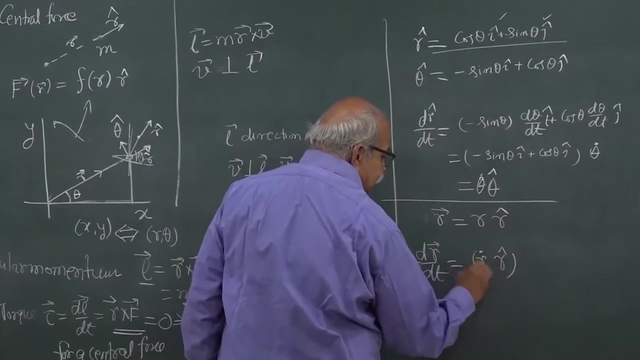 r cap. So what is d r d t, d r d t? this is the velocity of the particle. this is the velocity of the particle d r d t, r vector here. So differentiate this, keep this as constant. then keep this as constant, differentiate this and that is equal to r dot r cap, then plus. 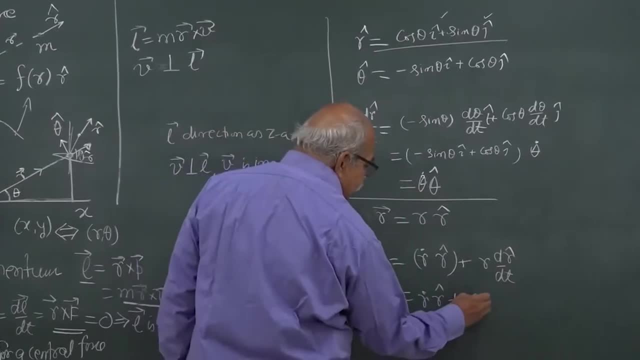 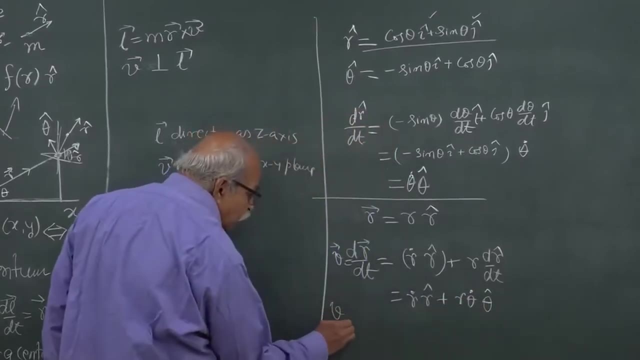 r times: d r d t. d r d t is right here, So it is r and then theta dot and then theta cap. So the r component is r dot and the theta component is r dot. So this is r dot. 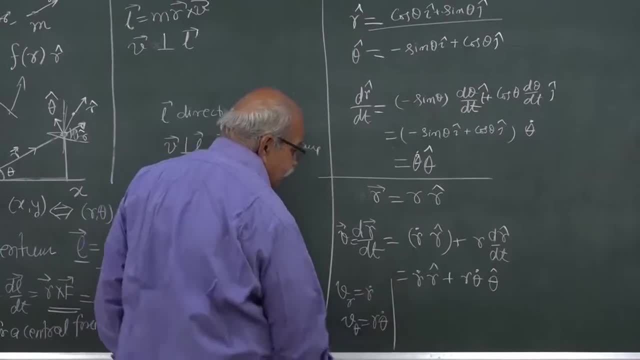 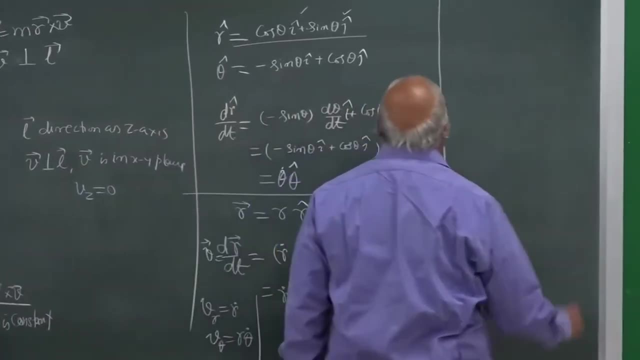 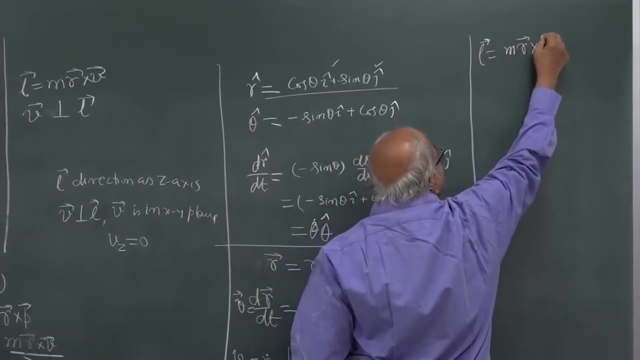 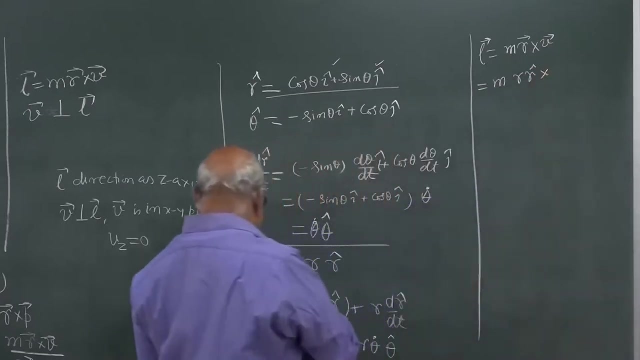 So this is r dot and then theta is r theta dot. you can write it like this: And you can write an expression for this l? l which is m times r vector, cross v vector and r vector is r r cap, and then cross v vector is here, v vector is here r dot, r cap. 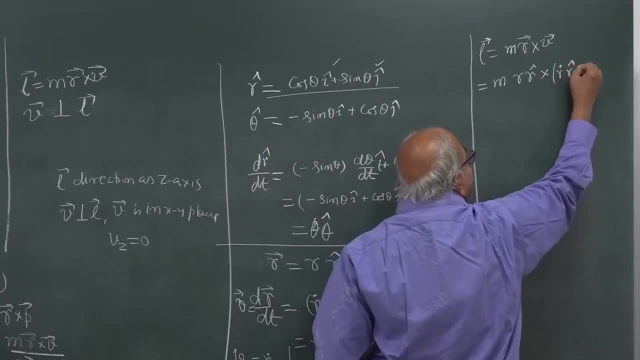 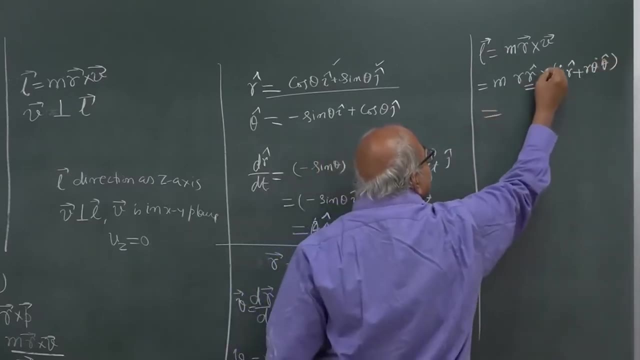 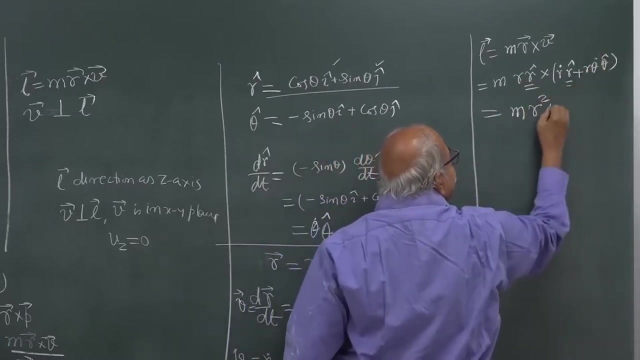 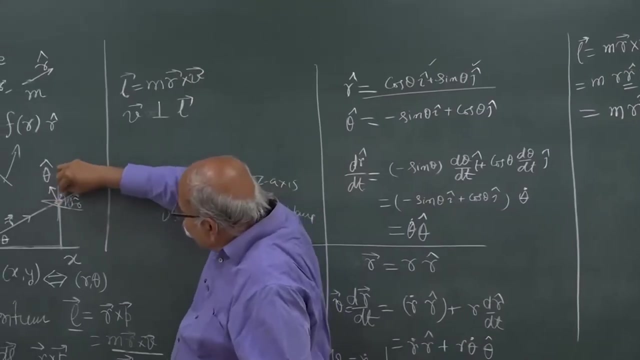 plus r theta dot theta cap. r cap cross r cap is 0.. So it is: m into this r into this r and then theta dot r cap cross theta cap. come back here. here is r cap and here is theta cap. So what is r cap cross theta cap? this is: